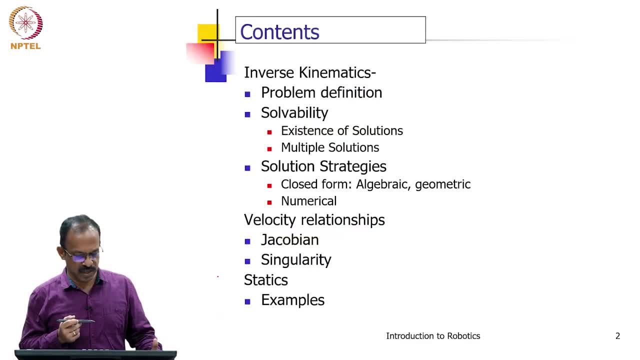 So what we are going to cover in this is basically the problem definition. So we will try to define what is the inverse kinematics problem all about, And then we will see something called solvability. So it is not that necessary that always the 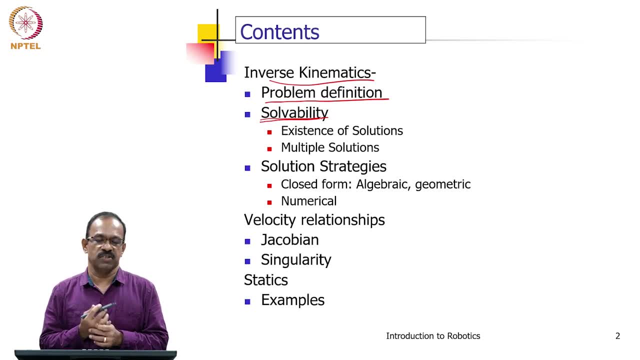 inverse problem can be solved. So it can be solved under certain conditions only. So we will see the existence of solutions and then the problem of having multiple solutions. So some cases there will not be any solution and some cases there will be multiple solutions. 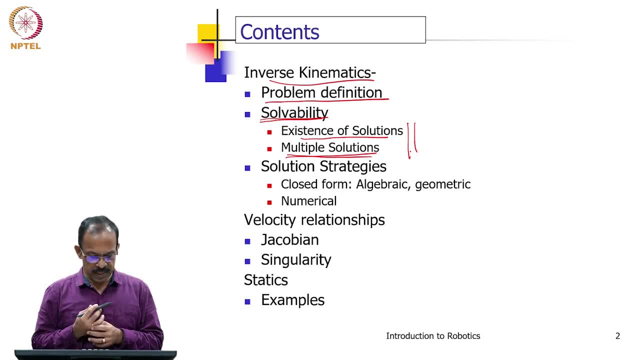 So we need to see what is that solvability? And then we look at the solution strategies. There are different strategies, Okay, So we will look at the close form solutions as an algebraic or geometric solution, And then we look into the. I mean, then there is another method called numerical solution. 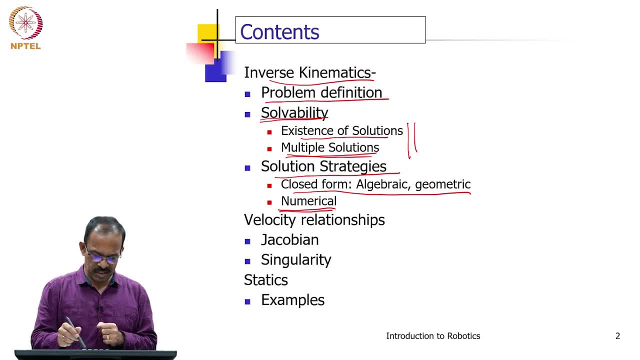 We will not go into the details of numerical solution, just for to tell you that that also is a method for solving inverse kinematics. But we will be talking only about the close form solution And then we go into the velocity relationship. Of course that is not the inverse. 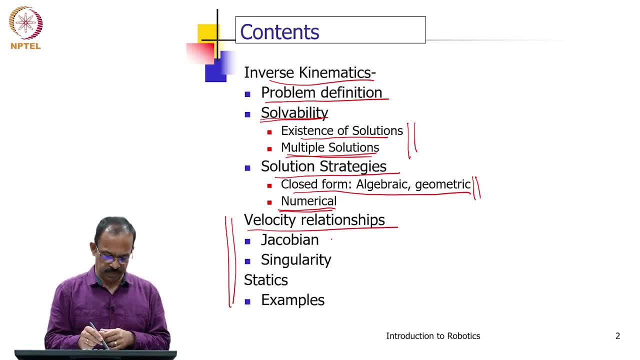 So we will look into the velocity relationship, that is, the relationship between the joint velocities and the tip velocities, where we discuss about the Jacobian and the singularity, and finally we will talk about the statics also, so the force relationship under static conditions. 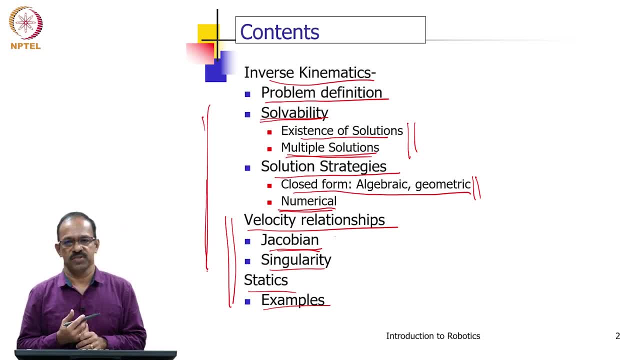 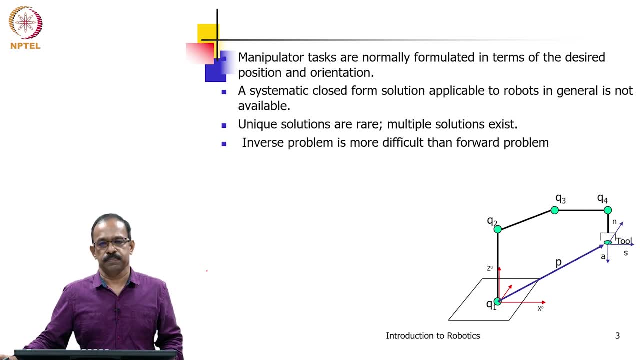 So that is going to be the discussion for the next few classes Now. we already mentioned about the inverse problem. what is the manipulator inverse problem? As you know, the manipulator tasks are normally formulated in terms of the desired position and orientation. 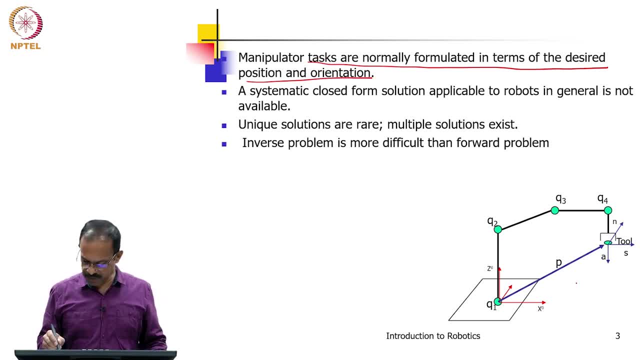 So, as I told you, so I have an object here, I have an object here, this is an object. Now I have a coordinate frame assigned to this object so that I know the relationship, position and orientation of the object with respect to the base of the robots. 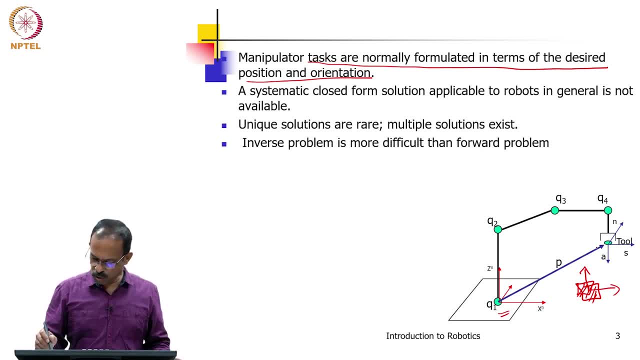 Now my interest is to see how can I use this robot to pick this object from here. I need to pick this object from here and place it somewhere here. I want to place it somewhere here and I know this position also, so I can define this position where I want to reach. 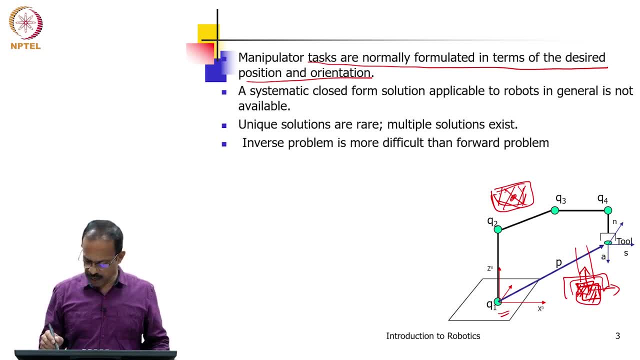 So I have this object in this position and I want to pick up this using this robot. So if I have to bring this tool to this position, what should be my joint angles is the in reverse kinematics. so that is the way normally all the manipulator problems. 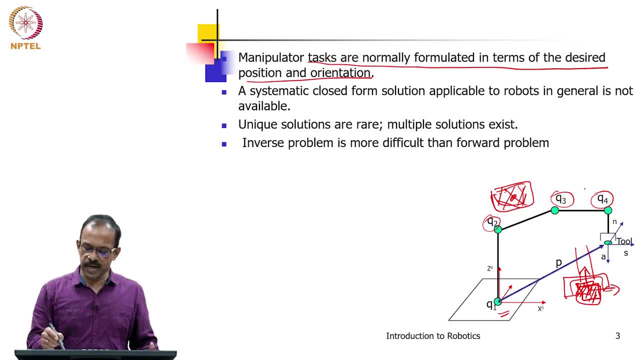 are formulated, So knowing the joint angle, and where to where will it reach the forward kinematics is useful, but not in the practical scenarios like this Here, So sorry. So here we are interested to know what should. 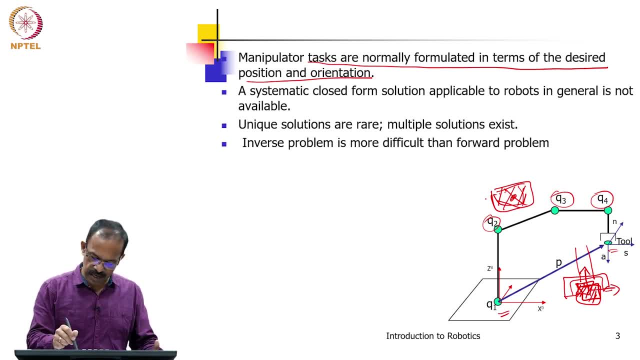 be the joint angles to reach here and, similarly, what should be the joint angles for the tool tip to reach here, to drop this point: object here: So that is what is the requirement in the practical application. So that is what says that they are normally formulated in terms of the desired position. 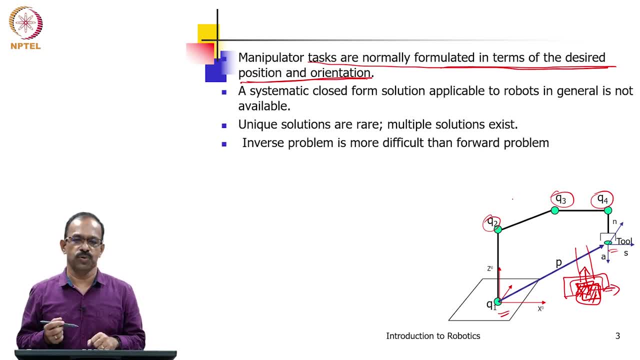 and orientation. So we have a desired position and orientation for the tool and we want to know how can I reach the? how can we reach that position and orientation using the joints? And that is the inverse problem that is of interest to us. So we have something from here to pick and then place it somewhere else. 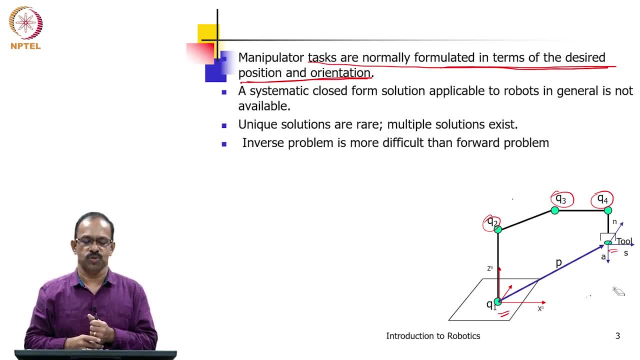 So how to reach these positions are the interest to us And a systematic closed form solution applicable to robots in general is not available. That is, this problem cannot be generalized because each robot will be having its own way of reaching that position And solving that problem. 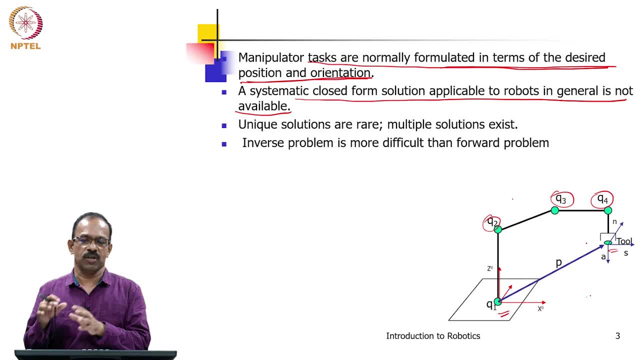 Position or getting the joint positions to corresponding to that position, cannot be generalized because of the robot configurations. We will see why the what the problem is later. but that is the problem here: it cannot be generalized, and unique solutions are rare and multiple solutions exist. 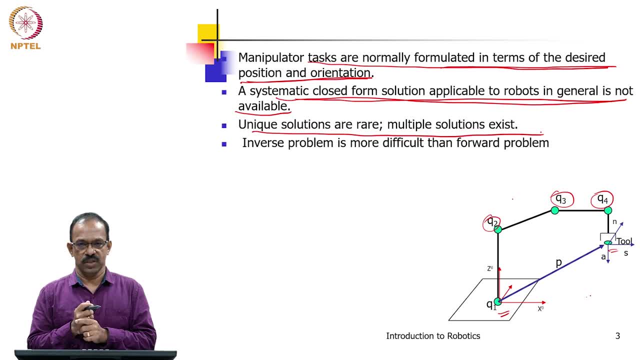 So many times you will be having multiple solutions that mainly because suppose you have a point here, Or assume that this object is here and you want to reach this point So you can actually reach from here, can actually reach from here and reach here, or you can actually 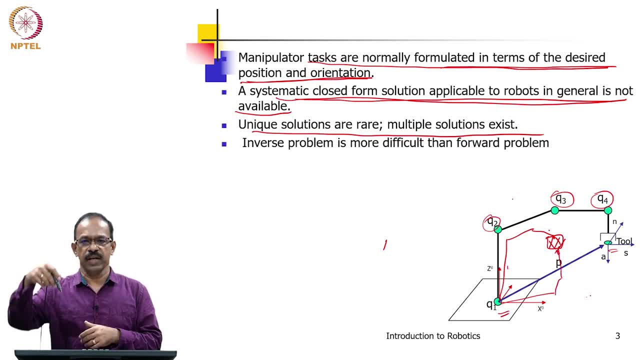 reach like this also, So you can actually have an elbow up or elbow down kind of a solution. So this kind of multiple solutions are very common, in inverse Okay, And because of all these You have this inverse problem as a very difficult than the forward problem. 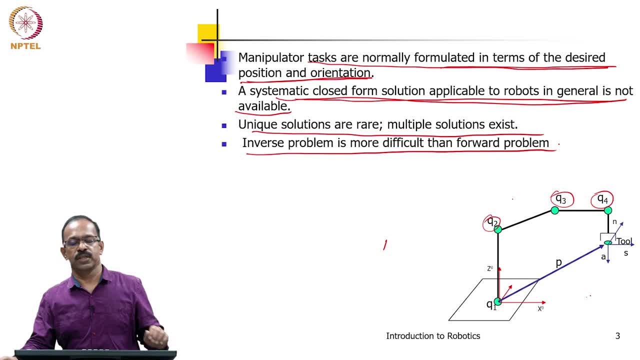 So forward problem was very generalized. for any set robot configuration we can have a general solution and therefore we are not able to we are able to get a generalized solution, But in the case of inverse, this is not possible because of various reason which we will see. 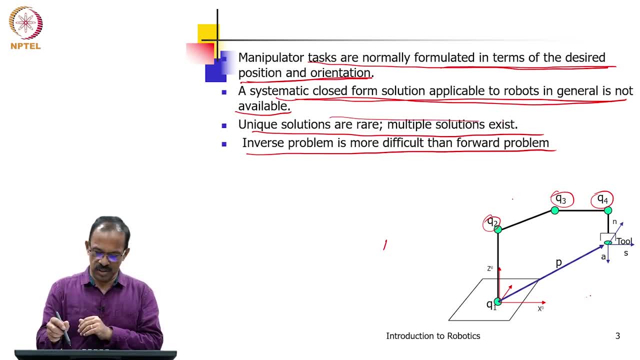 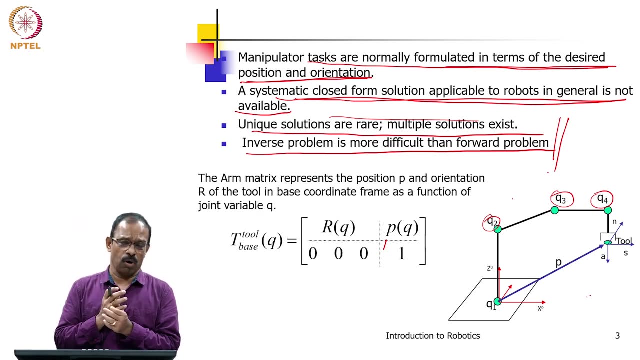 later and unique solutions are not there. So all these actually leads to, So the inverse problem as a complex one compared to the forward problem. Okay, So now if you want to solve this inverse problem so we can look at what is happening, 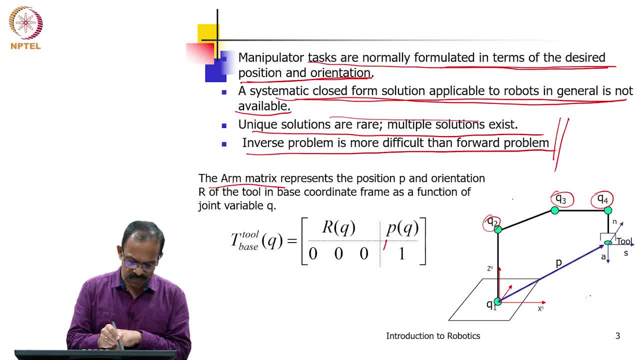 in the forward relationship. So we have this arm matrix which we discussed in the forward relationship, which represents the position p and orientation of the tool in base coordinate frame as a function of the join variable q. So now when we, So now when we. 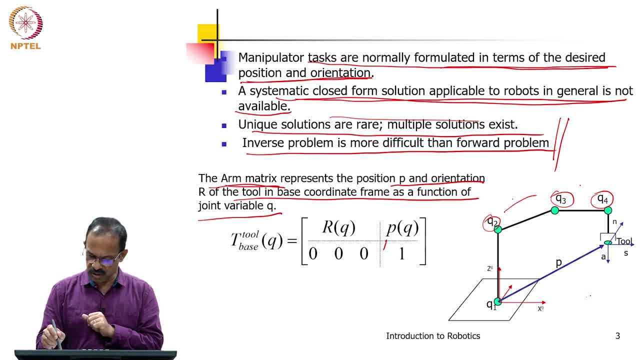 So when we do a forward kinematics, for q is the join variable here, so q are the q, the set of join variable, then we can actually represent the position p, So this position vector p and its orientation or the end of this tool frame can be represented. 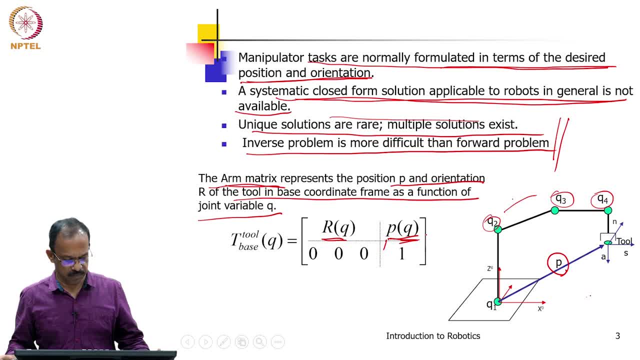 using this rotation matrix and the position vector. rq and pq rotation matrix and the position vector can be used to represent this. Now, what is this p? p is basically the position of this. So this is the position vector. So this is the position vector. 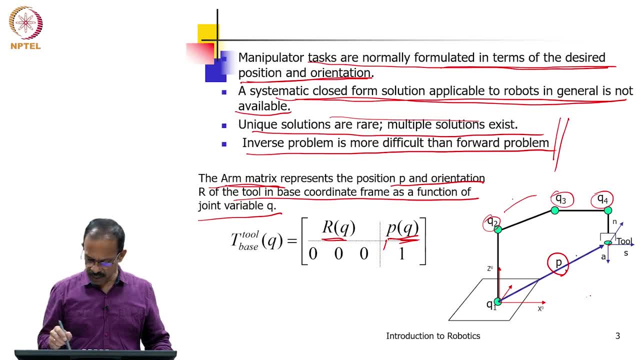 So this is the point position of this point p and represented in terms of px, py and pz. So we represent it as px py, pz and then we have a relationship: px is something, px py is something. 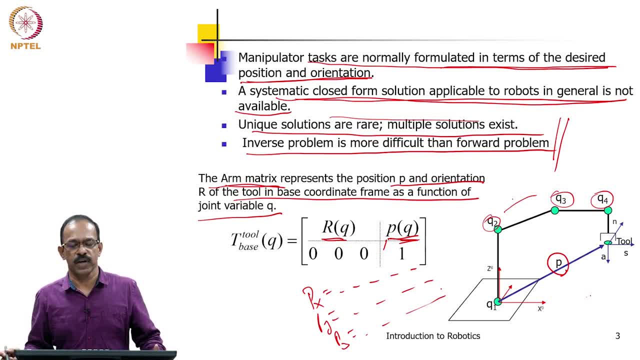 This is what we get in the forward relationship And this will be a function of the q. So we know that it is a function of q. depending on the type of robot, it may be a function of q1 to qn. 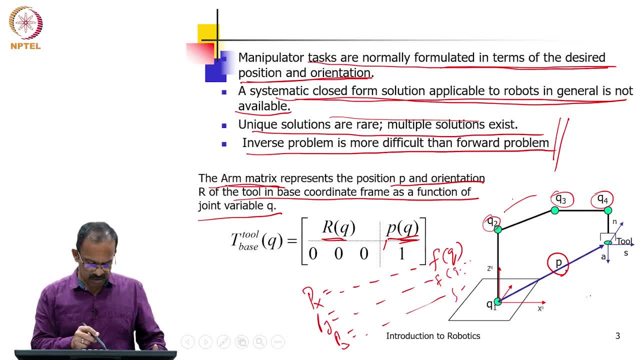 And this also is a function of q1 to qn. Similarly, r also. we have this as a vector. I mean 3 by 3 matrix. so you have the normal approach and sliding vector. so you can call it as nx, ny, nz, like that. 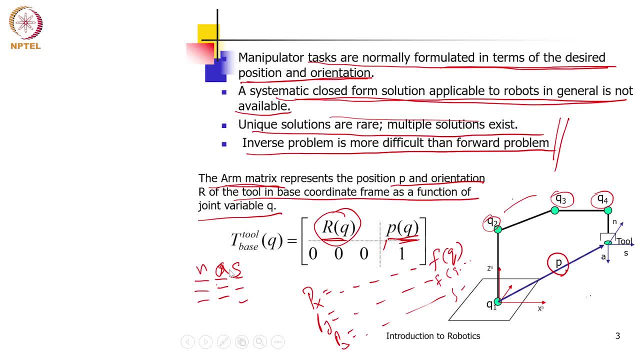 And each one also. we saw that this also is a function of joint variables. So nx is equal to nz, So nx is equal to nz, So nx is equal to nz. So nz is a function of joint variables. ny is a function of joint variables like that. 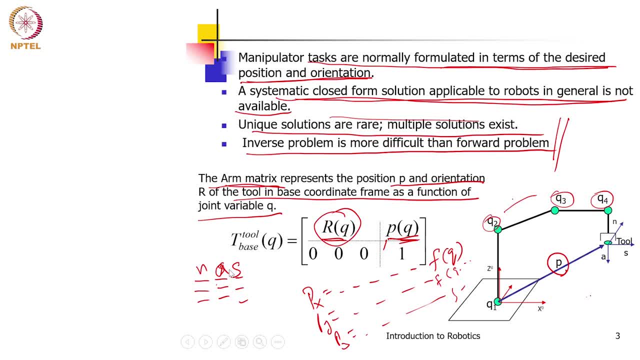 So we have these equations available with us. Now the question is: how can we actually use px? suppose we know px, how can I find q1, q2, q3? So we have to start from the forward relationship and then solve this relation to find out the. 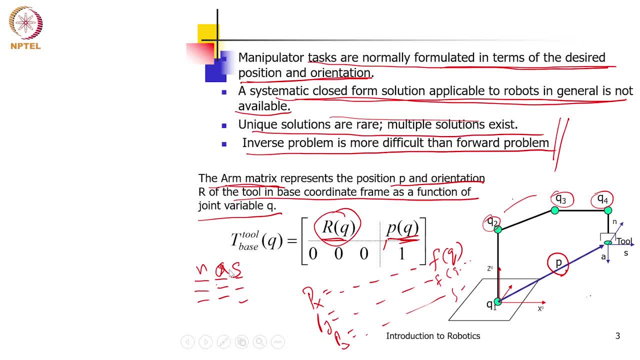 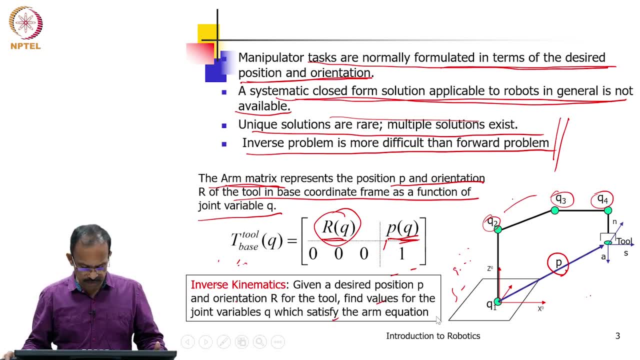 q. So that is the requirement in inverse kinematics. So, given the desired position p and orientation r, So these are the terms For the role of the tool: find values for the join variables q which satisfy the arm equation. 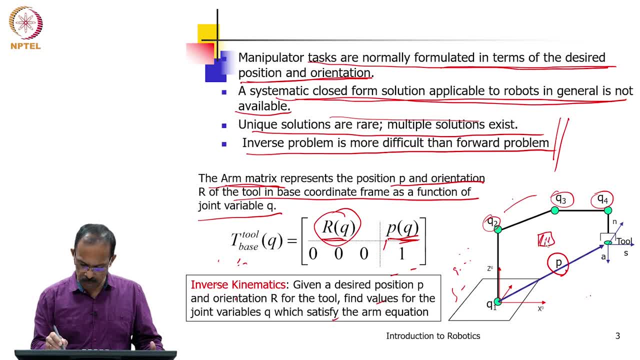 So now, if suppose this p is given to you, now you want this p to be reached. here you say that okay, this is the p which I want to reach. and I have an orientation like this: if this is known, if this p and this rq is known, how can I find this q corresponding? 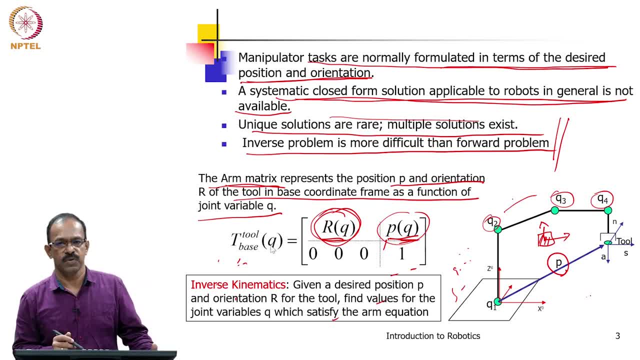 to this p and r. That is the inverse problem. So, given a desired position p and orientation r, So we are able to find the p and q All right. equation R for the tool: find values for the joint variables Q which satisfy the arm equation. 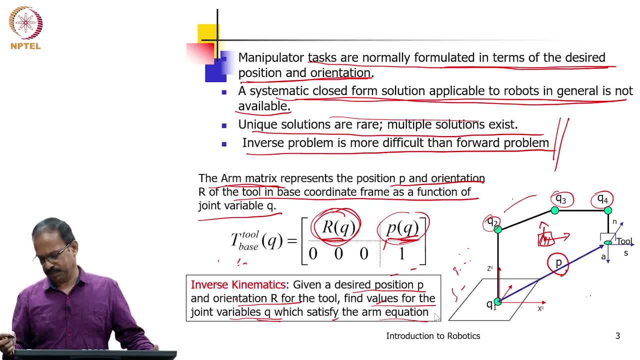 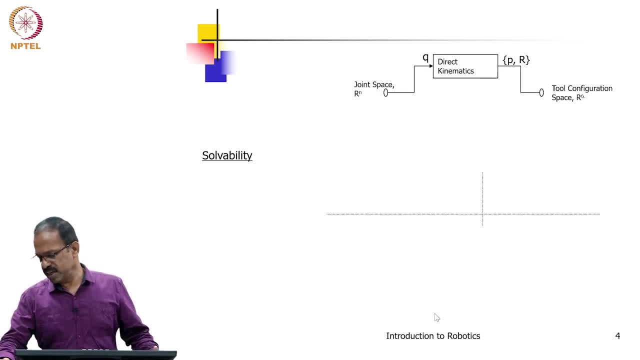 So this is the inverse kinematics problem. So to represent this relationship between the direct and inverse kinematics, you can see that if you have the joint space parameters Q, if you know this, Q1 to Qn, that is, we call the joint space joint parameter, joint variables. 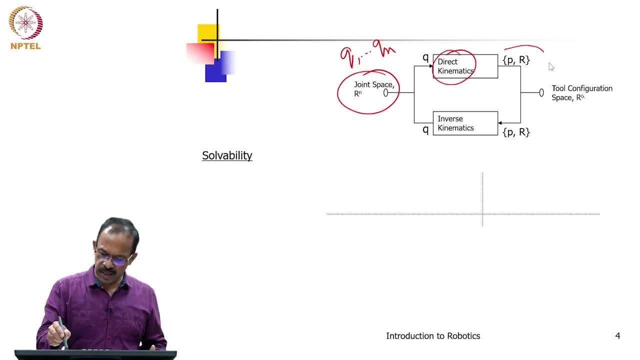 Now we use the direct kinematics or the forward kinematics to get the tool configuration space Rn, which actually is the P and R, that is, the position vector and the rotation matrix, can be obtained. So for any value of Q you will be able to get the position and orientation. 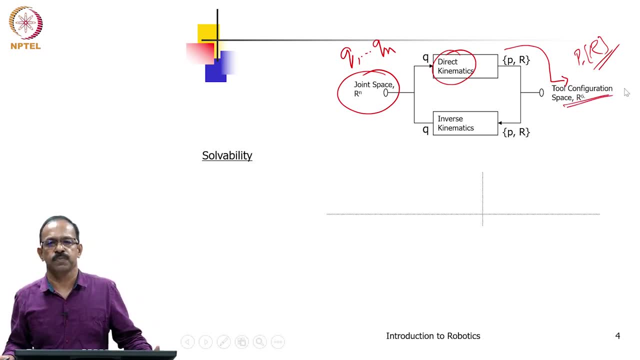 using the forward kinematics. we call it as a tool configuration space. So that is it, Thank you. Now, if you apply this inverse kinematics to this- suppose you have you know P and R- then you apply inverse kinematics and you get the joint space variables. So use this. 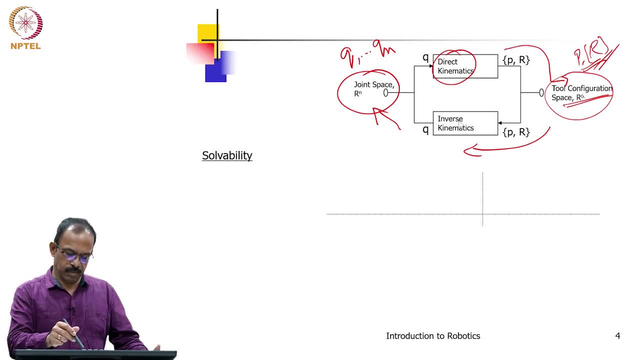 tool configuration space information using inverse kinematics. then get the joint space is the inverse problem. So you can see that if we want to solve the inverse kinematics we need to have a direct kinematics relationship, In that directly kinematics relationship is the one which is used to solve the inverse. 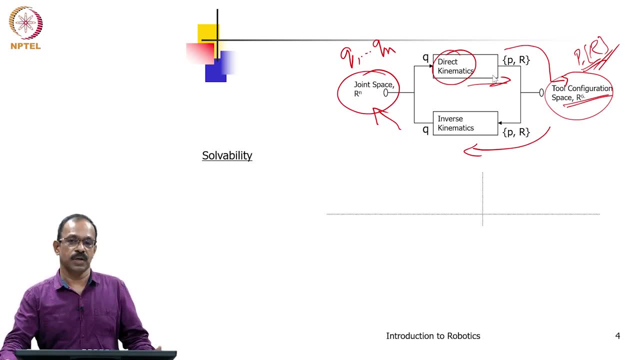 kinematics problem or we need to know the forward relationship of the manipulator to solve the inverse. kinematics and the arm matrix should be known to us. So now look at the solubility of this relationship. So, as we know, if you P and R are known, then 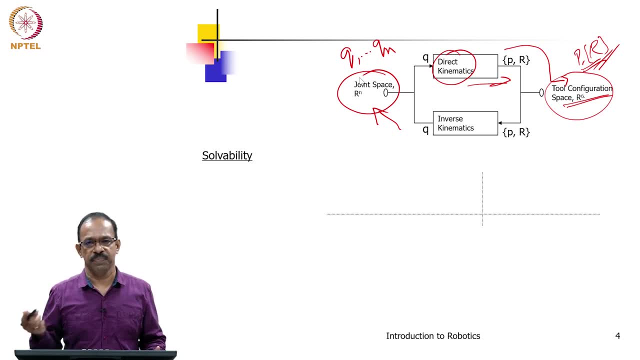 we can use some method to solve for Q. So that is the inverse requirement. Now see and R are represented. Suppose we have this relationship for the arm matrix. it says that px, py, pz and nx, ny, nz, sx, sy, the normal sliding and approach vectors- normal sliding. 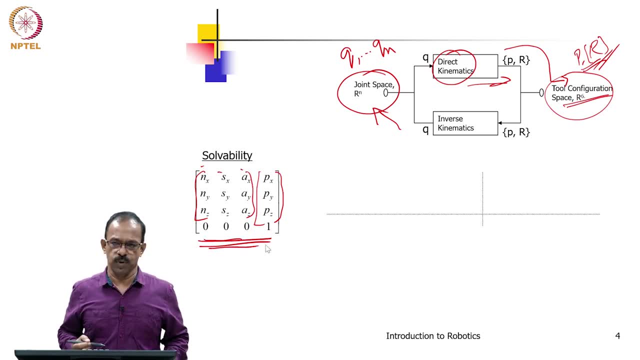 and approach vector and the position vector is the one which is given to us because we assume that we know this or this is known to us and we want to solve for the joint variables which corresponds to that one. Now, in the case of normal case of forward kinematics, how is it represented, This px? 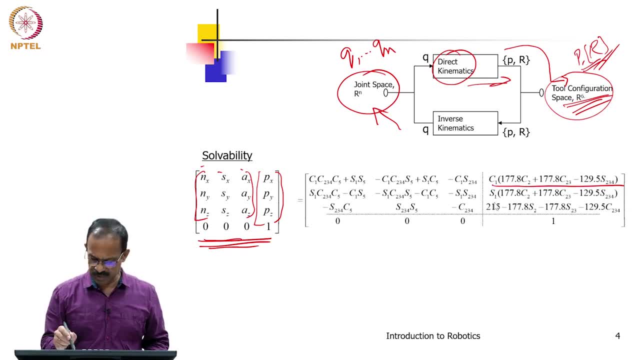 py- pz will be represented like this, For example: I have taken one robot configuration and for that robot we will see that px is equal to this one and py is equal to this one and pz is equal to this one. So we can see that there can be three relationship. 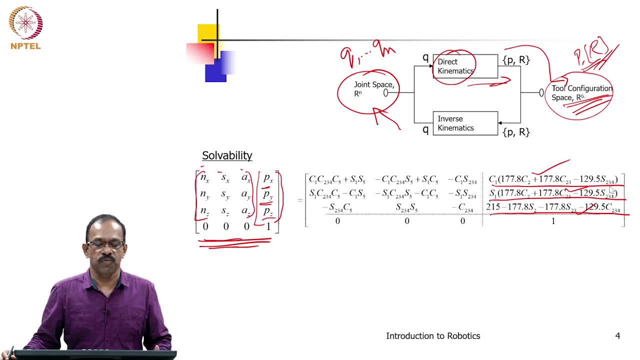 three equations can be written for that particular manipulator. We have a relationship that is that px is equal to c1 multiplied by something, py is s1 multiplied by something and pz is 215 minus something- something. So that is the three equation that you can have. 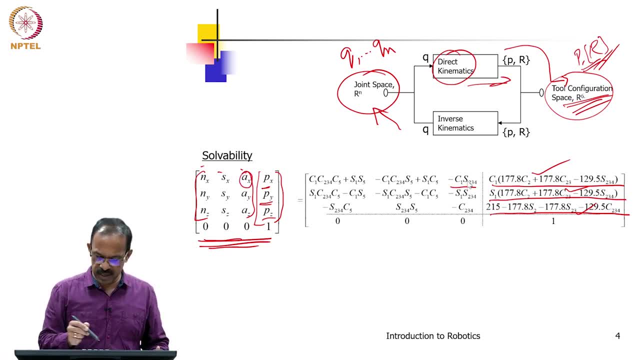 Now, similarly, we can write: ax is equal to minus c1, s2, 3, 4,. ay is equal to minus s1, s2, 3, 4,. az is equal to minus c2, 3, 4.. So like this, we will see that we can actually. 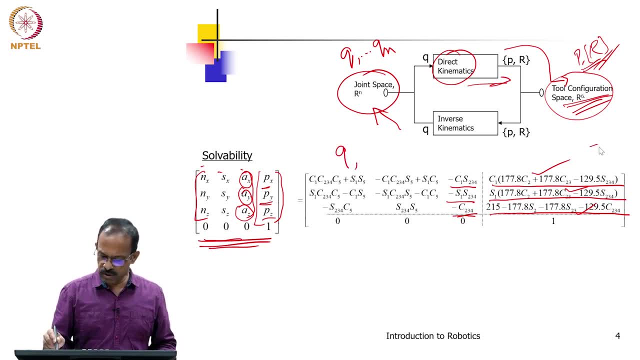 get nine equations from here and three equations from here, So we have totally 9 plus 3, 12 equations from this matrix relationship. So arm matrix is given. so for px is equal to this, py is equal to this. like this, we have 9 plus. 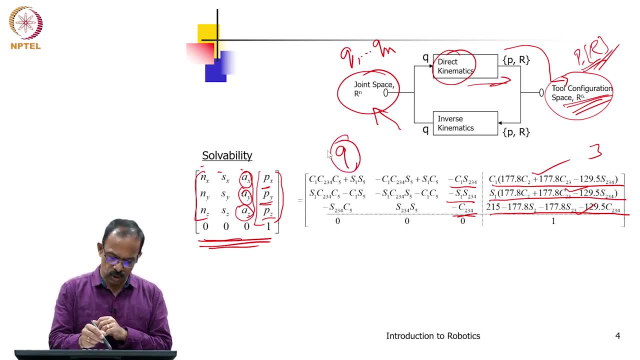 3, 12 equations And using this 9 plus 3, 12 equations, we need to find the joint variables q1 to qn. So you have q1 to qn to be formed. Okay, I will show you the last also, how to. 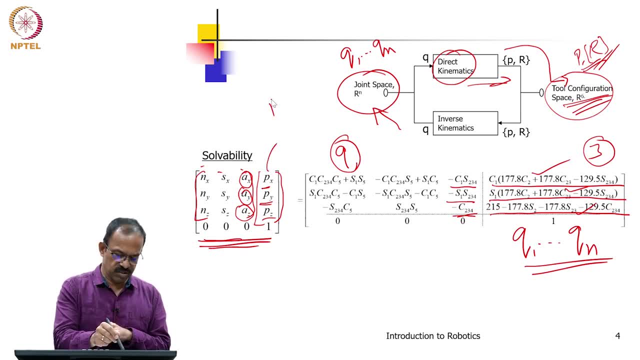 found out, because if px is given, suppose I have- px is equal to 170 and py is equal to 50 and pz is equal to 50. Now I have to write 170 is equal to this, 50 is equal to this and 50 is equal to this and solve it to find out what will be the values of theta. 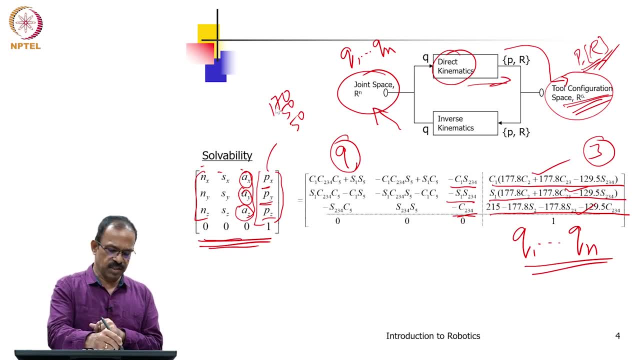 1, theta, 2, etcetera, which satisfy this condition. So that is the way how we need to look at this. So we have 9 plus 3, 12 equations and n unknowns. n may be 6 or 5 or whatever it. 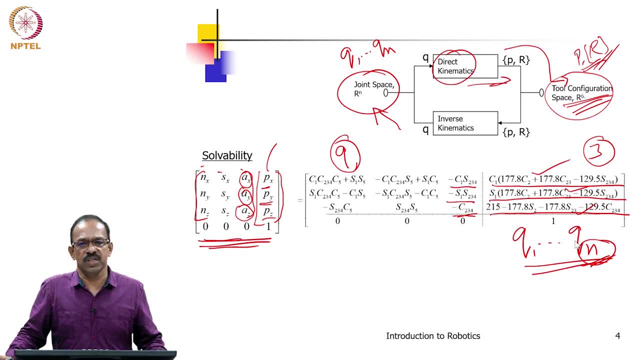 is. So we will see that there are 12 equations and you have n unknowns to solve. So things seems to be simple, because you have 12 equations and you have only n unknowns. this n will be normally 6 or 5 or whatever it is. 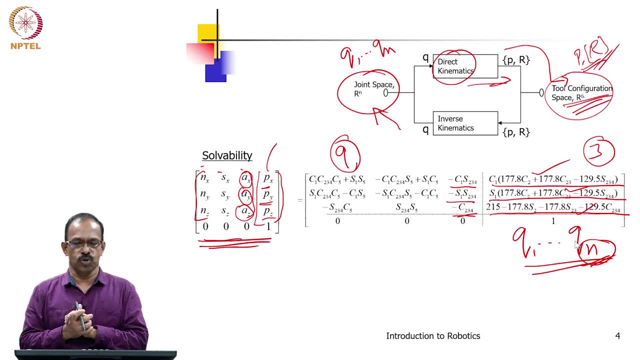 So that seems to be a simple equation. So this is a easy problem to solve. But if you look at closely this one, you will see that there are 12 equations and n unknowns and 6,, 4, 6 axis robots. But if you look at 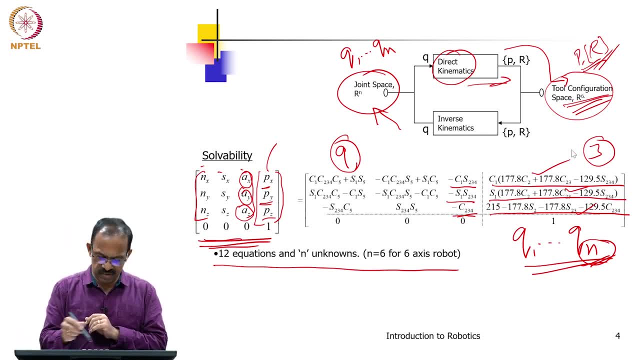 closely this, these three equations, we can say px py, pz. they are independent because you can actually place the robot in the position. the end effector can be placed anywhere in the x, y, z plane within the workspace So that it can be independent. So px py, pz. 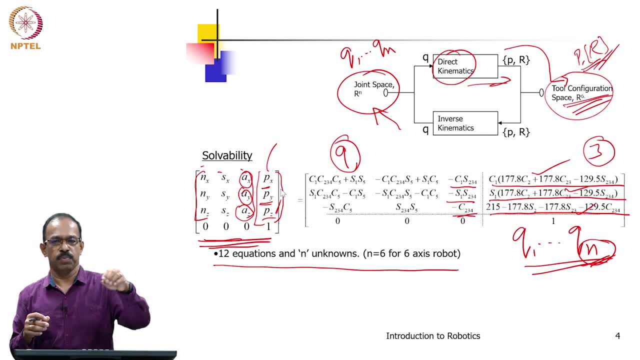 there is no relationship directly. as long as where you want to place it, you can place, So you can actually get. these three equations are independent. They have three independent equations here, But these nine equations, they are not independent. The reason is that 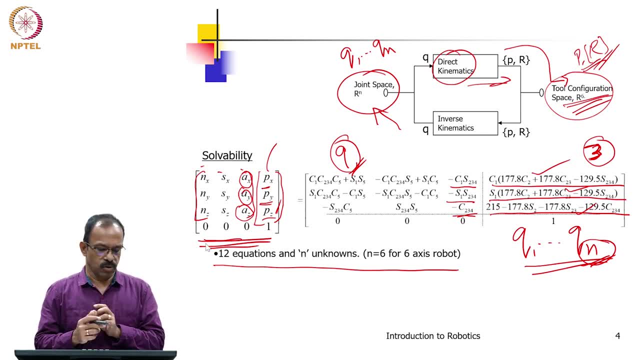 this actually represents three vectors. So this actually represents the normal vector, sliding vector and approach vector and they are orthogonal and, of course, they are independent vectors. But these three out of these, nx, ny, nz- they are not independent. There is a relationship. 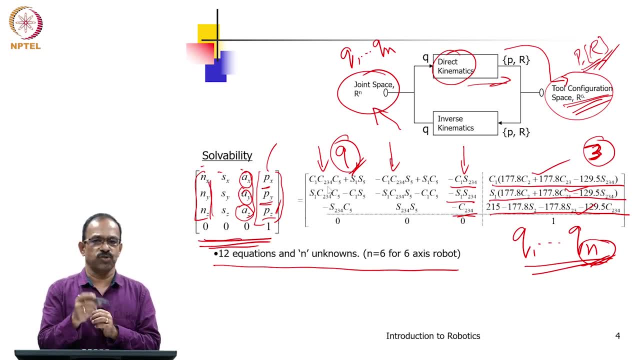 between nx, ny and nz to satisfy this condition of the vector. So nx square plus ny square plus nz square is equal to 1.. Similarly, sx square plus sy square plus nz square is equal to 1, and ax square plus ay square plus az square is equal to 1.. So that is the unit. 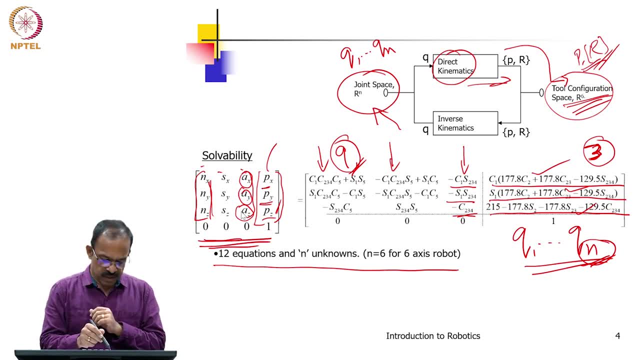 vector, the three orthogonal directions. So these three equations that you see here, you are seeing here, these three equations are not really independence And similarly, these three equations are not independent. These three are not independent. So effectively we have only one equation from here which is independent, and this is only one equation. 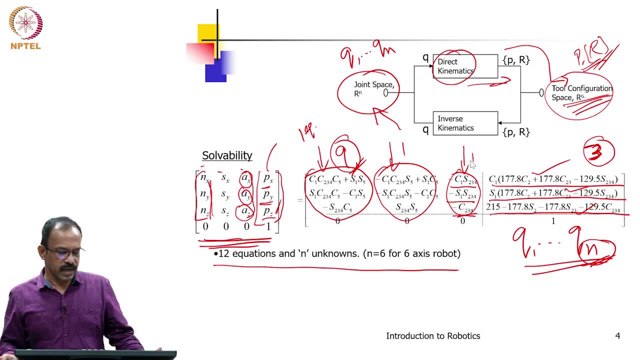 from here and this one equation here, So we can have only a three independent equations from the rotation part. This rotation matrix gives you three independent equations, though we have nine equations, since they are not independent. So in Egyptians they are split into thousands, acred�. So 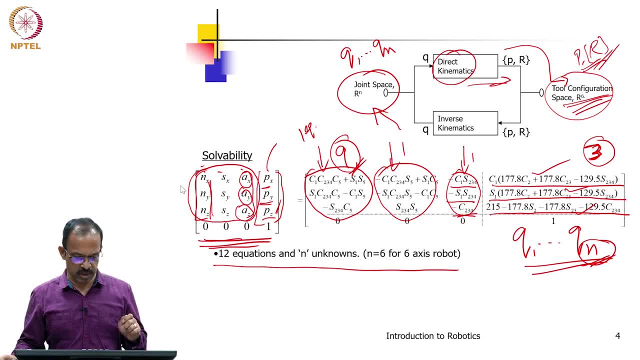 independent. what we can see is only 3 independent equations. So these 3 independent equations from this part and then 3 independent equations from the positioning part, give you totally 6 equations. So you can actually get 6 independent equations from the arm matrix. So using the 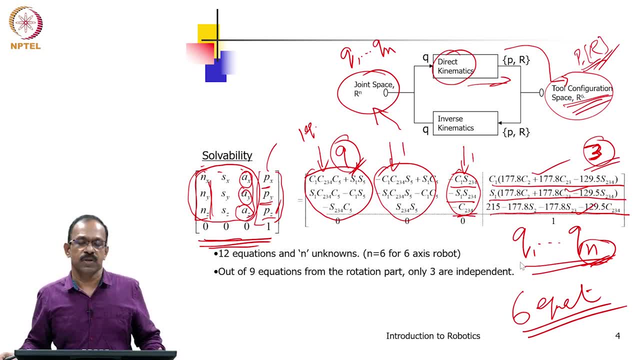 arm matrix you will be able to get 6 independent equations to solve for the n variables, So 6 equations. now we have n variables. So if the n is equal to 6 or less than 6, we can solve the problem. But when n is equal to 7, you will not be able to solve because 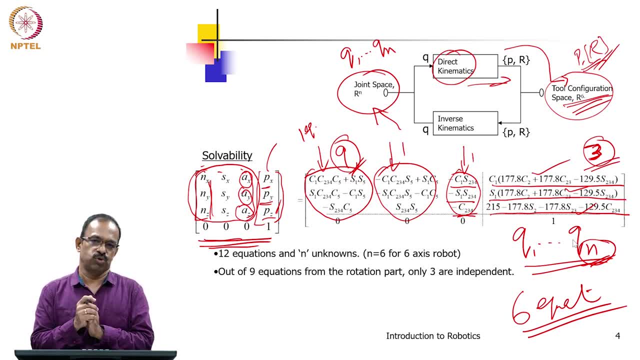 you have only 6 equations and 7 unknowns cannot be solved, So you need to choose one of these. you have to select, and then you have to get other 6. So that actually leads to multiple solution, depending on the values of the first assumption. 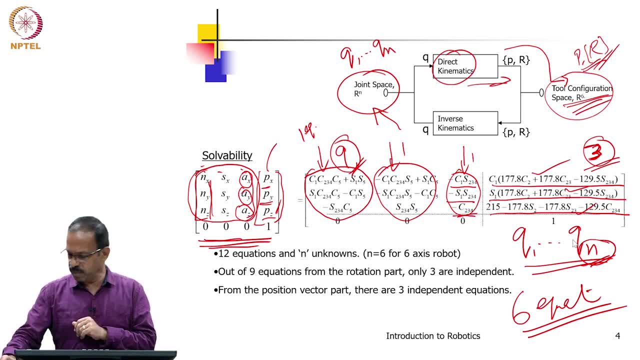 So effectively we have Only 3 independent equations and 3, 6 independent equations and n unknowns and nonlinear. they are nonlinear equations and then difficult to solve. So 6 independent equations and n unknowns and nonlinear equation. So we need to solve them in order to get find out. 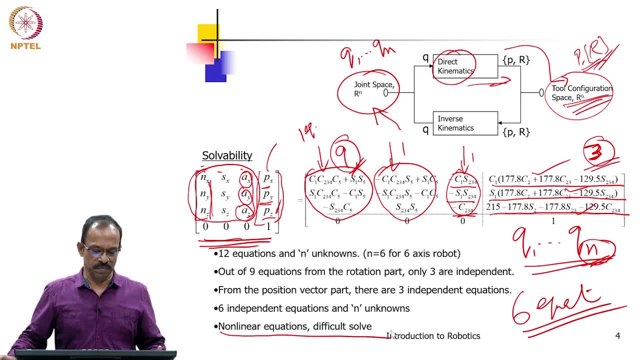 the joint variables. but they are not that easy to solve because they are nonlinear equations and n is more than 6. again you will have. So you have to get n unknowns and then difficult, difficulty. So that is the difficulty with the inverse kinematics, or that actually tells. 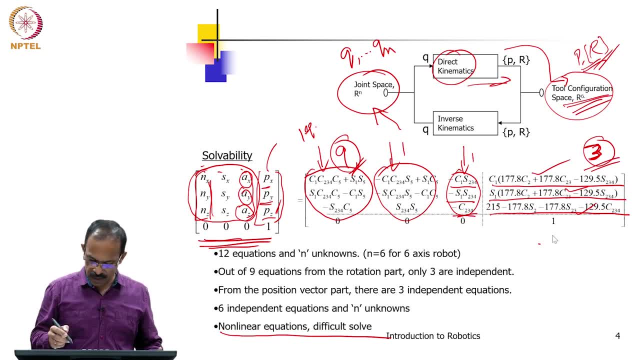 you the solvability aspect of the inverse problem. We have six independent equations and n unknowns and the relationships. what you are seeing here are the nonlinear equations and not that easy to solve. Now we have to see how to address this problem for manipulators. 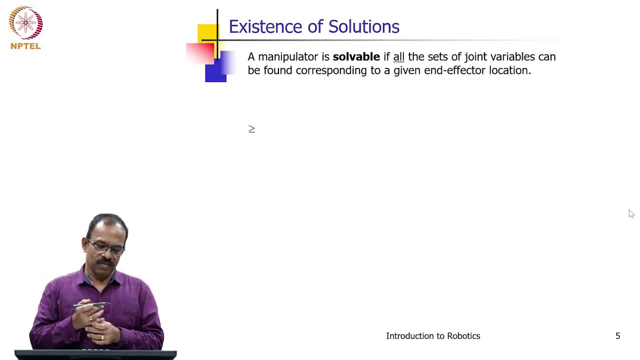 So first thing we look at this: is there a solution existing or not? So we know that there are six equations and six unknowns. suppose it is 6, n and n is equal to 6.. So we have 6 equations and 6 unknowns, so we can actually solve the equations, that is. 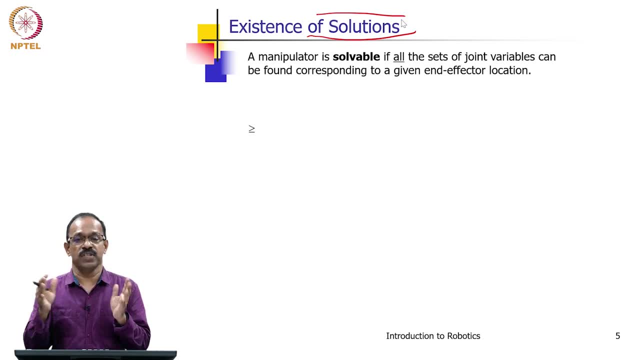 possible, but whether there is a solution existing or not, if there is a solution existing, then only we can solve it. So if we have to solve using the 6 equations, first thing we need to do is that in this case, you have to solve it. So what you do is that you can. 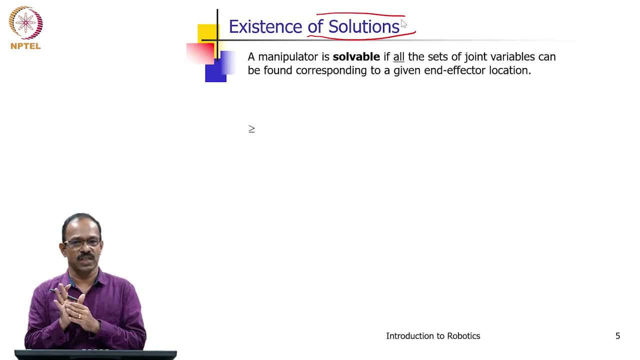 need to ensure is that, yes, there is a solution existing for it and therefore start solving it. And how do we ensure that there is a solution existing? So we look at this a manipulatory, solvable if all the sets of joint variables can be. 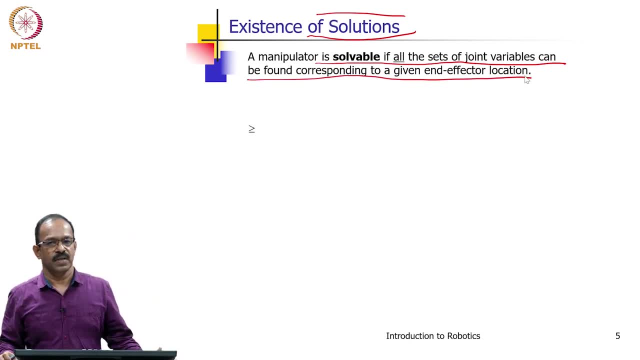 found corresponding to a given end-effector location. So a location is given to you and if you can find the all the joint angles corresponding to that location, then we call it as a solvable one. That means you need to get all the sets of joint variables which can actually reach to. 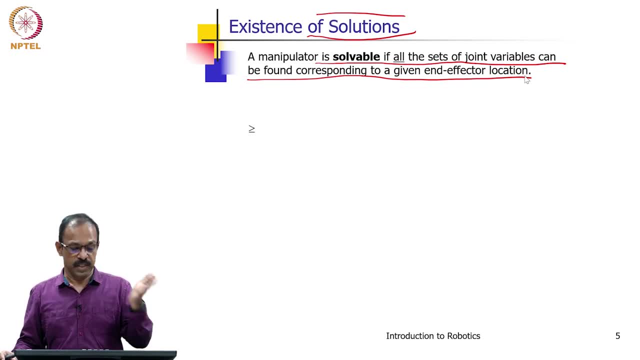 that position and orientation. So then if we can find it, then we call it as a solvable. Now there are few conditions under which we can say this is possible. So not all positions are solvable and there are some position which cannot be solved. also, 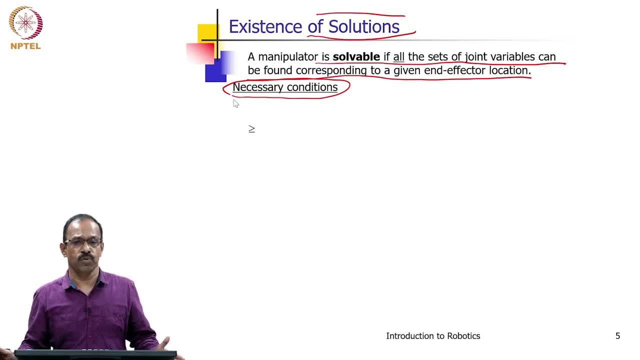 So first we look at what is the necessary condition to have a solution. That is, if you want to have a solution, what is the minimum condition to be satisfied? What is the necessary condition to be satisfied? The first point is that suppose you have a robot like this, suppose this is the robot. 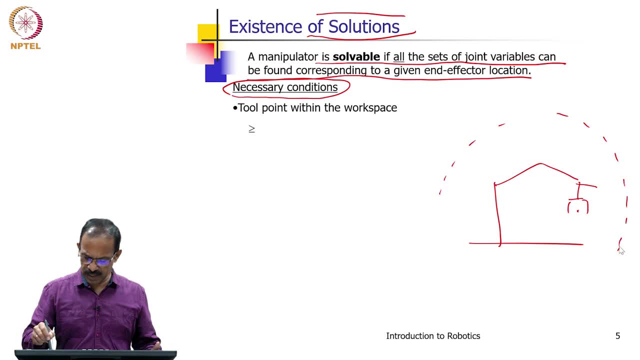 and I will say its workspace is something like this. I am just roughly mentioning. this is the workspace that the robot is Now as a programmer. I may not be knowing that. what is the workspace it can reach or what is the all the points. 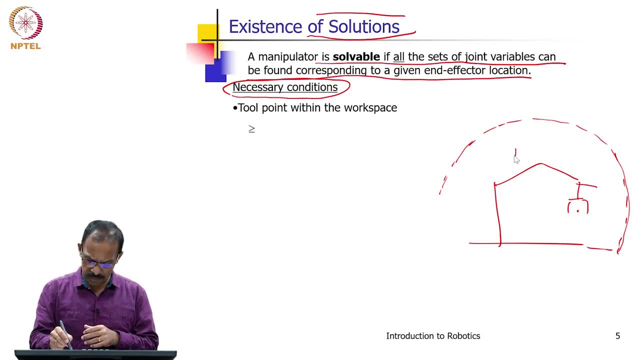 I may not be knowing. Suppose I give a position here, maybe it may be possible to solve, But if I say that I want to reach this position, then it is definitely not possible to reach this position because it is beyond the workspace of the manipulator. 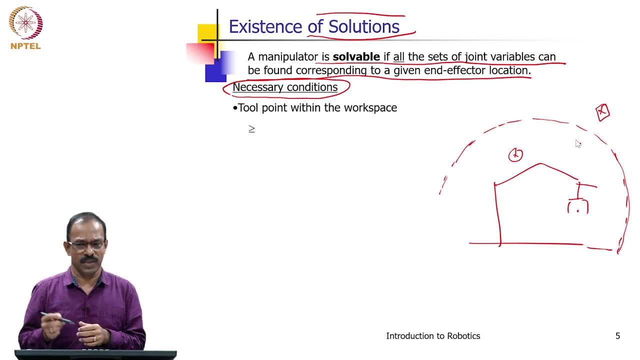 So the necessary condition to have a solution is that it should be within the workspace. That is, without that condition you cannot, never, can never solve the problem. So that is the first point. So first condition is that the tool point within the workspace. 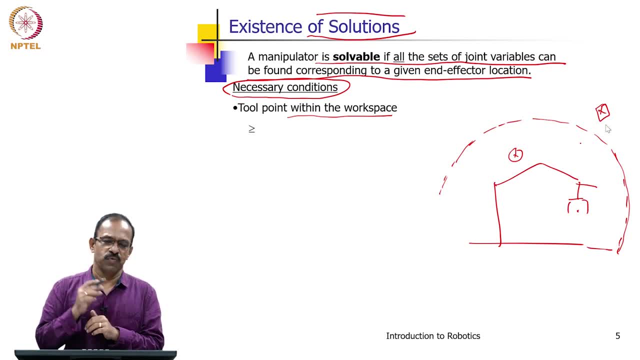 So the tool point, what you have want to solve, should be within the workspace. that is the first condition. Now we know that if I want to reach this position, I will be able to reach this position, and if I want to get a particular orientation also. so I need to have a orientation desired. 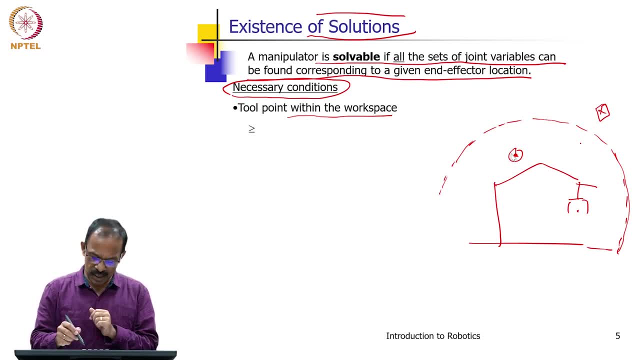 orientation at desired position, then I know that there should be three degree of freedom for positioning and I need to have another three degree of freedom for orienting. That means I can get any orientation and any position within the workspace using this three plus three degree of freedom. that is six degree of freedom. 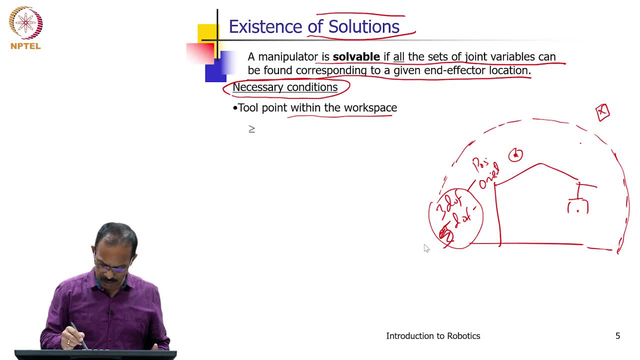 Suppose I have only five degree of freedom, suppose I do not have. I mean I have only five degree of freedom, then it is clear that I would not be able to reach the orientation needed. I can use the first three degree of freedom to reach the position. 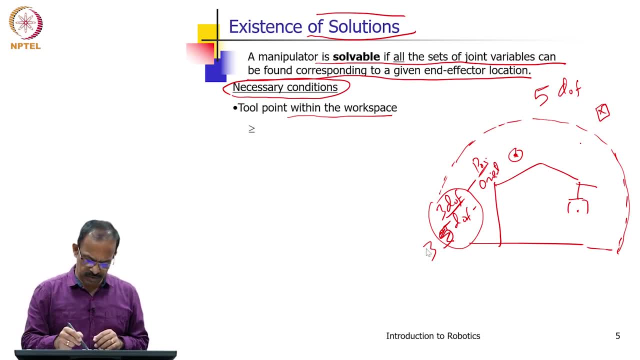 So that is the first point. But then I have only now left with only two degree of freedom out of five, three used for positioning. so I have only two degree of freedom for orientation. That means I would not be able to get all the orientations. I can control two orientation. 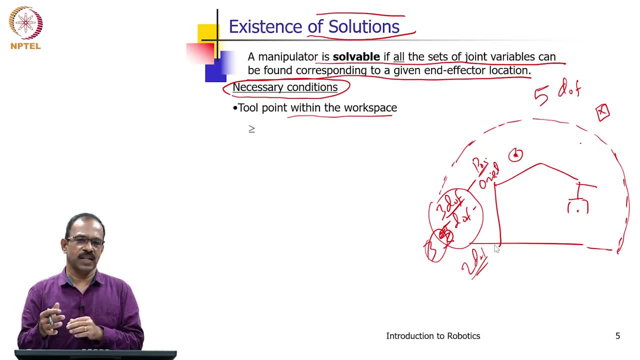 and the third one will be depending on the two. So I cannot really say all the three orientations I want and then only have only five degrees of freedom. it is not possible. then you would not be able to solve. So that is the condition: if n is greater than or all 6, to have any arbitrary orientation. 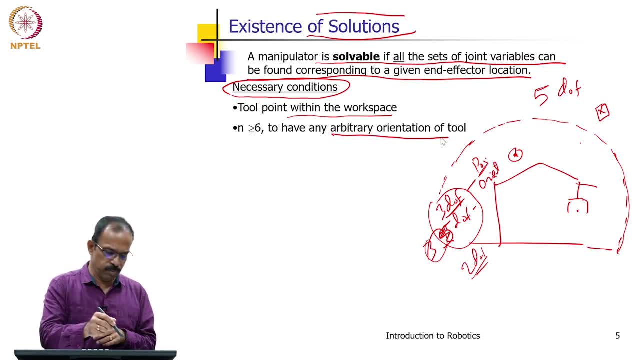 If I have to have any arbitrary orientation of the tool, I need to have minimum six degrees of freedom or more than 6 degrees of freedom. So if n is equal to 6 or more, then I can have all the arbitrary orientation, and if 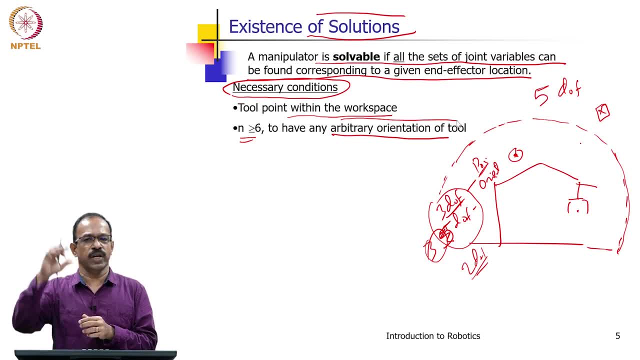 I have only five degrees of freedom, then then I say that I need to get all the orientations. it is not possible. that means I will not be able to solve for any arbitrary orientation if there is a there is only five degrees of freedom or number of degrees of freedom. 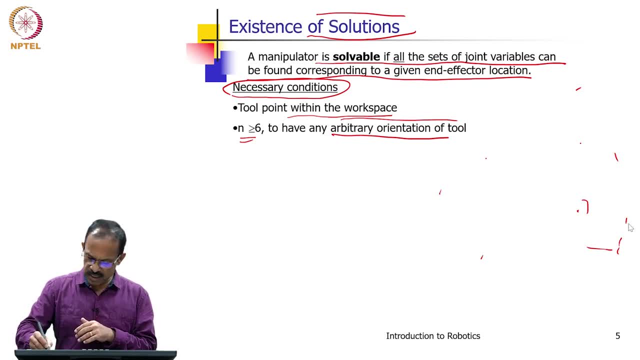 is less than the three, less than 6.. So that is the second condition, necessary condition to have the solution. So first condition is that the tool point should be within the workspace. The second condition is that n should be 6 if I want all the orientations achieved. 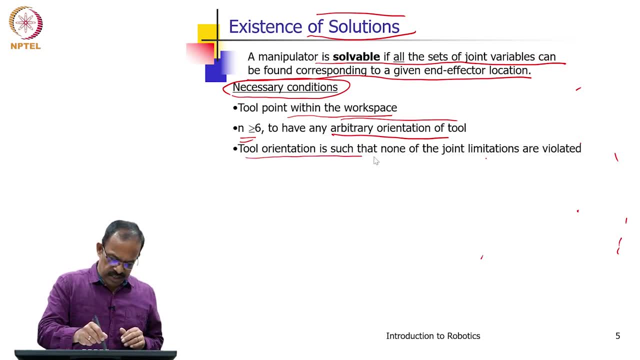 Now, another condition is that the tool orientation is such that none of the joint limitations are violated. So all the physical, all the robots will be having some physical limitations in joint movements. So whether your wrist will be having roll pitch and yaw axis and 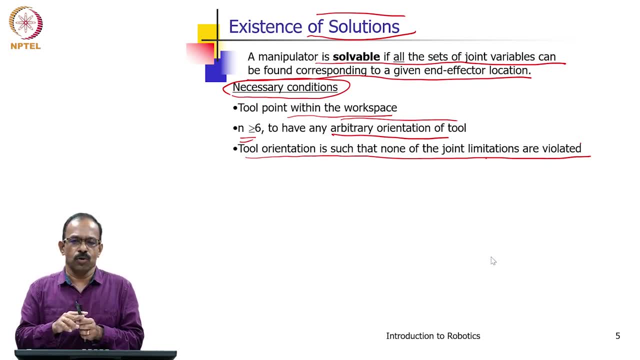 each one will be having some joint limits. So maybe roll can have all the 360 degree but pitch and yaw cannot have a 360 degree rotation because of the physical limitation. Now, if your orientation says the orientation, what you want actually can be achieved, if 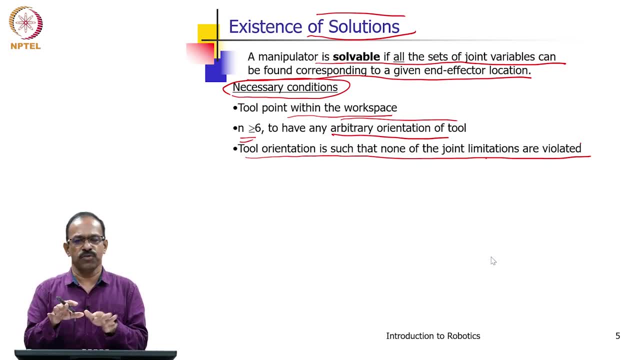 the joint limitations are violated, we will be getting a solution. But if you say that the joint has limits, then you will not be able to get the all the desired orientation. So we need to ensure that the tool orientation is such that none 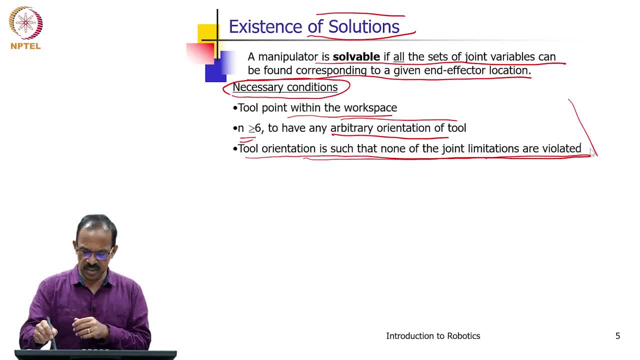 of the joint limitations are violated. So in these three conditions, these three necessary conditions to be satisfied if you want to get a solution or to have a to make the manipulator solvable, Now that is the necessary condition. So there are two kinds of solutions. One: 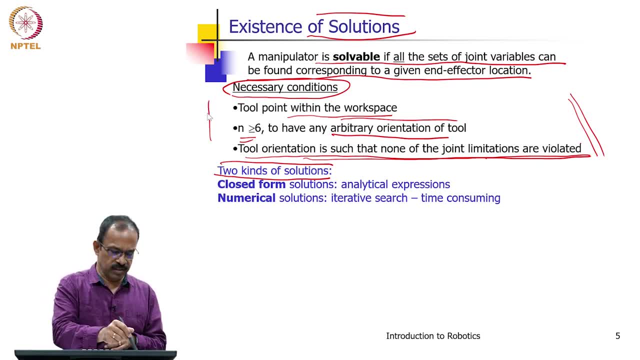 is the closed form solution and the other one is numerical solution. So closed form solution is that you can use the algebraic expression or the analytical expression that you already developed using forward kinematics. So you can use these analytical expressions and solve for it. 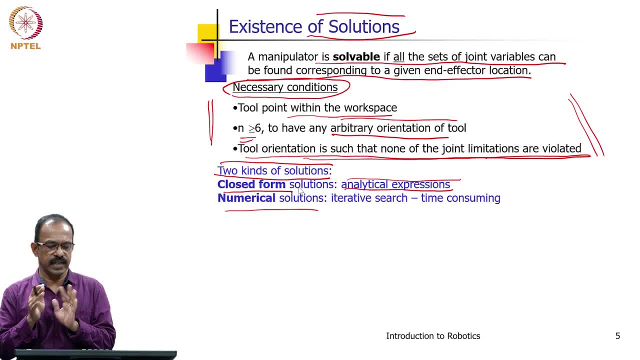 4: closed form solution. So the analytical method can be used to get a solution. then we call it as a closed form solution. So analytical method can be either these equations or you can have a geometrical method also. So two methods are there. either you directly solve. 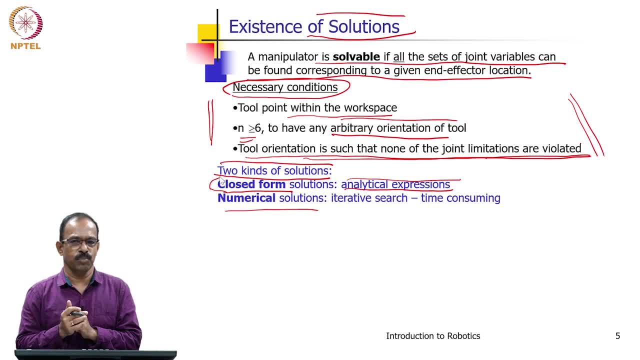 this algebraic equations, or you go for a geometrical approach and then find out the possible joint angles which will provide the position and orientation. So that is the closed form solution And the other one is known as the numerical solution, where you do an iterative search. 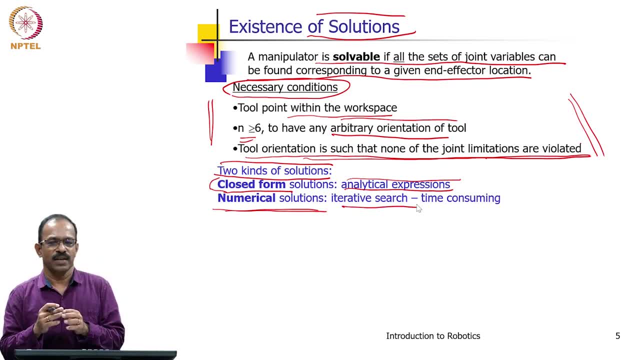 and then find out the solution. So you start with some value for each joint angle and then search all other joint angles which will actually lead to the desired position and orientation. And if you do a search and at some point you will find that, okay, how this meets the requirement. 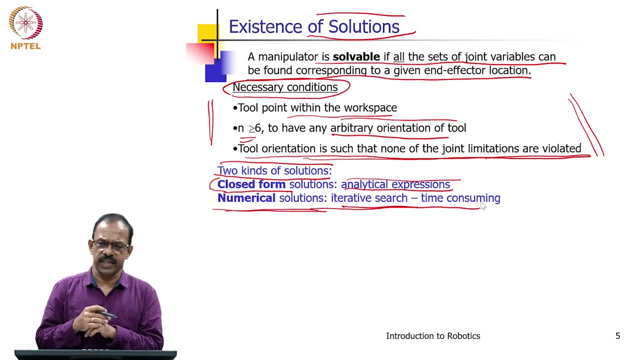 So that is the numerical method. So that is the numerical method, which is an iterative and time consuming method. So whenever the closed form solution is not possible, we have to go for time consuming method of numerical solution. Similarly, when you have large number of degrees of freedom, you have 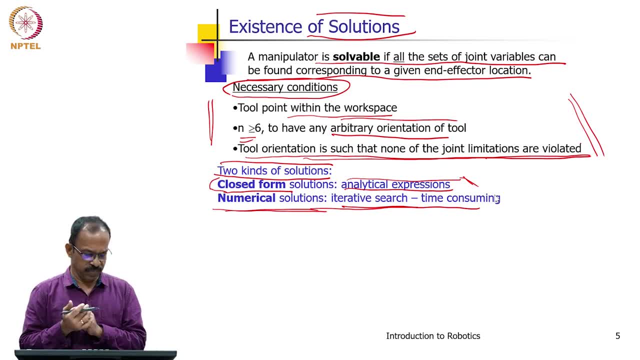 multiple solutions, then also you may have to go for a numerical solutions to get a most feasible solution. So how do we know whether there is a closed form solution existing or not? That is the second question. So the first question was that whether it can be solved or not. Now, if it can be solved, 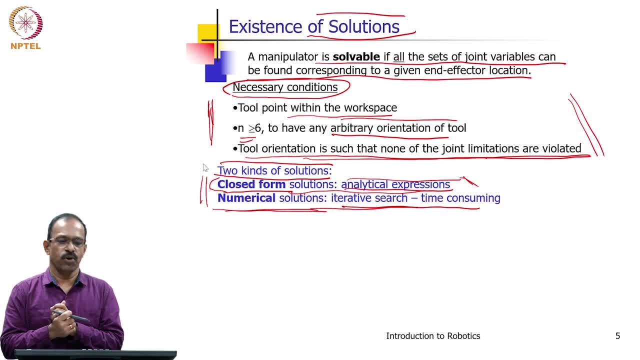 which method to be used. We will go for a closed form solution or a numerical solution And to get this closed form solution we call there is a sufficiency condition. We say that there is a sufficiency condition to get a closed form solution. So any manipulator 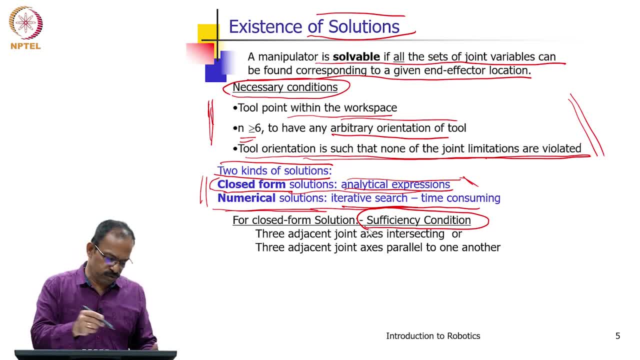 can be solved for its inverse using closed form methods. If it is agile, it can be solved. So any manipulator can be solved for its inverse using closed form methods If it is satisfy the conditions given here. that is known as the sufficiency condition. 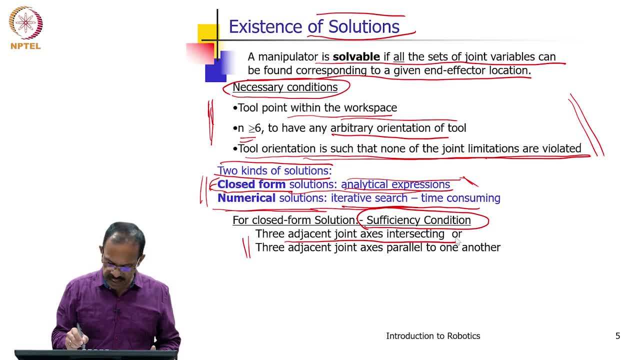 Sufficiency condition says that if three adjacent joint axes are intersecting, or three adjacent joint axes are parallel to one another, then we will be able to solve the inverse kinematics using the closed form methods. And if this condition is not satisfied, then you would not be able to solve it using closed. 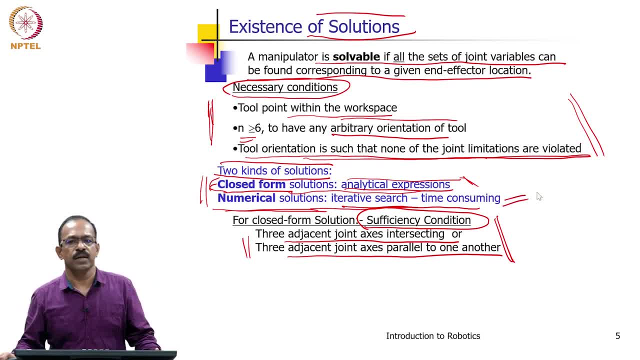 form methods, You need to go for a numerical methods. that is the situation, or that is the condition that says sufficiency condition where you can solve this using closed form methods. And what does it says? So suppose you have this axis like this: you have one axis here, one axis here and one. 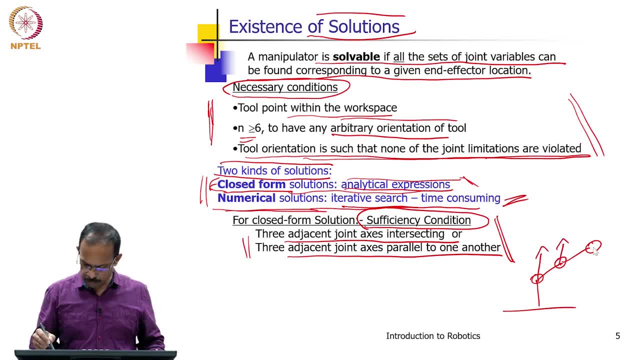 axis joint here and all the joint axes are parallel, Then you can solve this. All the adjacent joint axes, so all the adjacent joint axes, all the three adjacent joint axes are parallel. then you can have a closed form solution. Otherwise, if the three adjacent joint axes, suppose you have one axis here and then one- 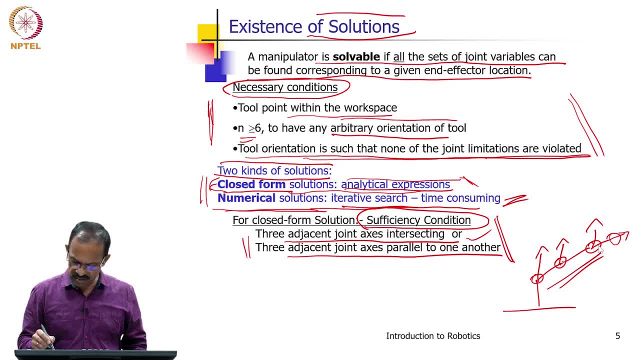 axis like this and one axis at this point which actually again intersect the these three. Suppose you have one axis and another axis here which actually like this, then these three axes are intersecting. If the three adjacent joint axes are intersecting, then you will be having a closed form solution. 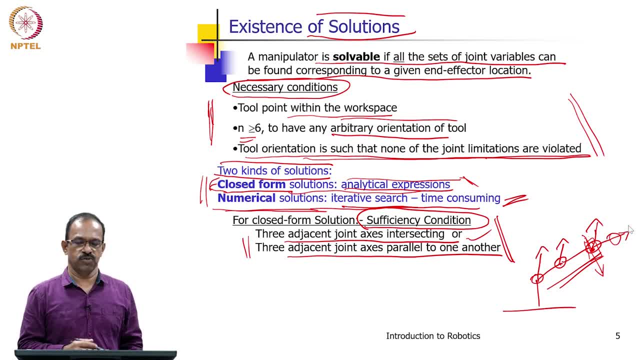 So this is the necessary sufficiency condition to get a closed form solution. So whenever you get a manipulator to be solved for inverse kinematics, first thing you need to check is whether the closed form solution is existing or not. If the closed form solution is not existing, then you would not be able to solve it using. 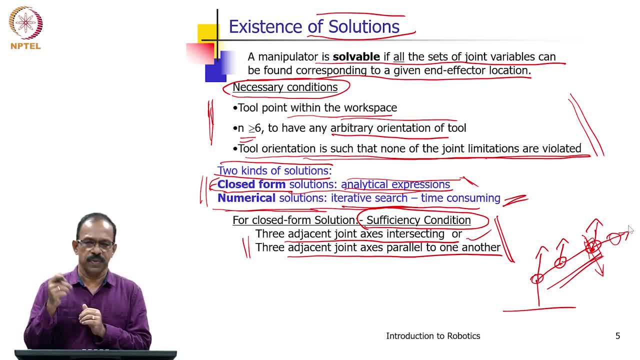 algebraic or geometric methods, You have to go for numerical method only. Okay, And from where this condition comes, that you can actually see later when we try to solve. So probably, if you remember the forward kinematic relationship, if there are three adjacent 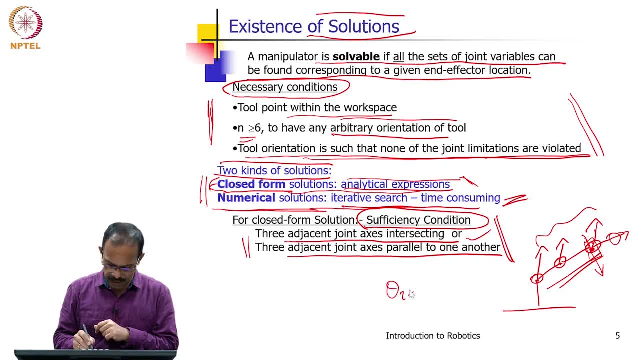 joint axes. you might have seen that it actually comes like theta 2 plus theta 3 plus theta 4 format, or we write it as theta 2, 3, 4.. So that is the form it was coming in, the arm matrix or the arm equation. 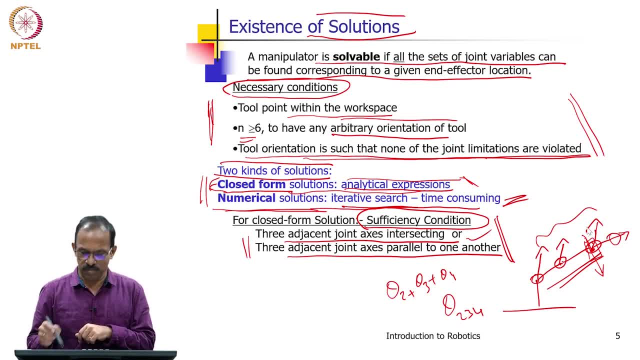 And that is the reason why we need to have this kind of parallel axes, So that you will be getting it in this format, So it can actually be solved. If they are not this way, then you will be getting 2, 3 and then theta 4 as another one. 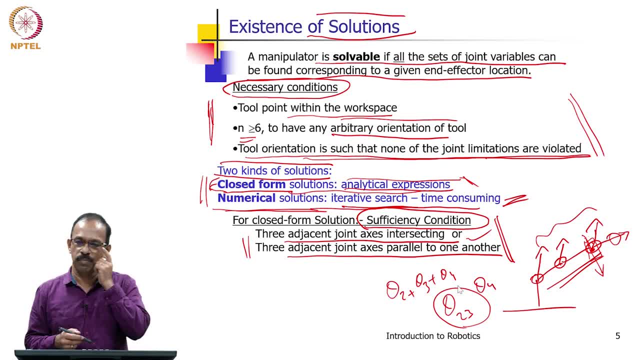 Then you have to solve for 2, 3 and 4 separately. that actually leads to problem in the solution. So this will be more clear when we try to solve the equations. but the relationship comes from this, this condition comes from that relationship. 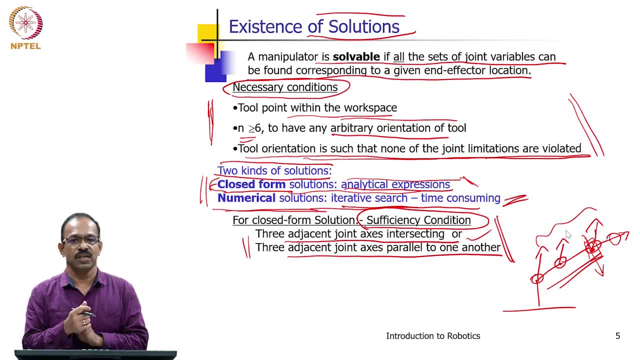 Okay, So that is the reason why we need to develop, or that actually happens in the forward kinematics. Similar is the case with the intersection, also intersecting the joint axis. Okay, So these are the necessary and sufficiency condition for getting the solution. 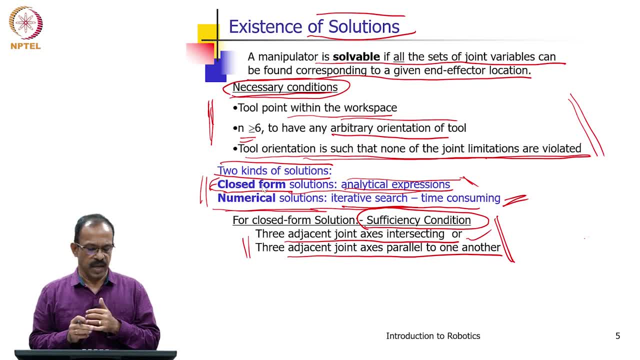 So necessary condition for existence of solution and sufficiency condition for existence of closed form solution. Okay, And as I mentioned, there will be multiple solutions. So when it is a redundant robots, so when you have n is equal to 7 or more, then we 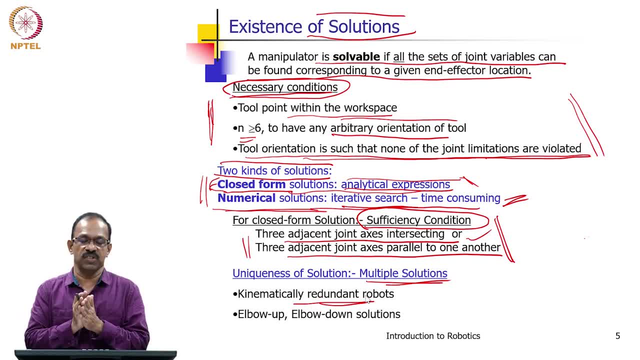 call it as a redundant robots, because what we need in space is 6 degrees of freedom, And if you have more 7 degrees of freedom or 8 degrees of freedom- controllable degrees of freedom- then it becomes a redundant robot. So whenever the robot is redundant, then you have multiple solutions, because you can only 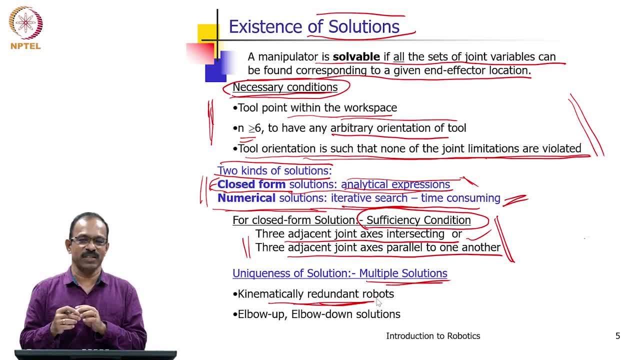 6 only you can solve So 7,, 8 and all. you need to make assumptions and then for each value of theta 7 or theta 8, you have to find for theta 1 to theta 6.. So that actually leads to large number of multiple solutions. 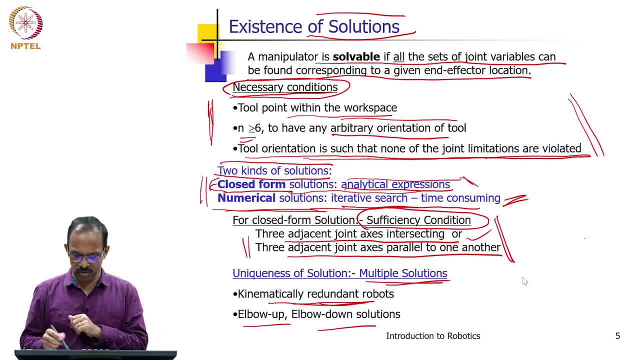 And another one is the elbow up and elbow down solution, which I already mentioned. So you have an elbow up solution like this, So you can actually reach this position from here, or you can actually reach the position from here. Okay, This is the elbow up or elbow down solution. 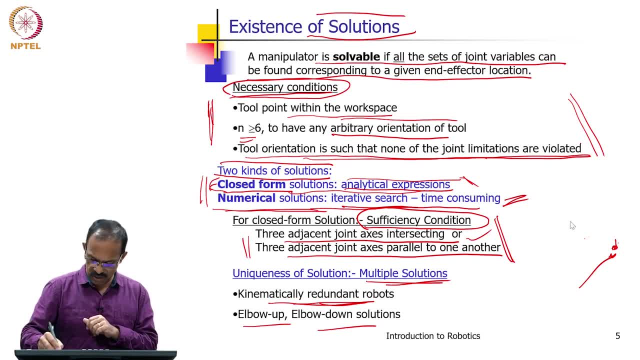 Okay, That also leads to multiple solutions. Okay, so always there is no unique solution. you will be, most of the time, you will be having multiple solution for the inverse problem. Okay, that talks about the basic requirements for the system to be solvable. 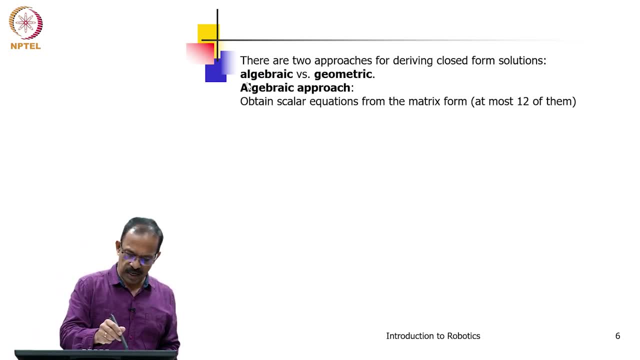 Now, as I told you in the closed form solution, algebraic and geometric approach is there. So the algebraic approach approach is obtained, That is obtained, the equations from the matrix, So the 12 equation that we already mentioned. So obtain the matrix equations, the scalar equation from the matrix and then try to 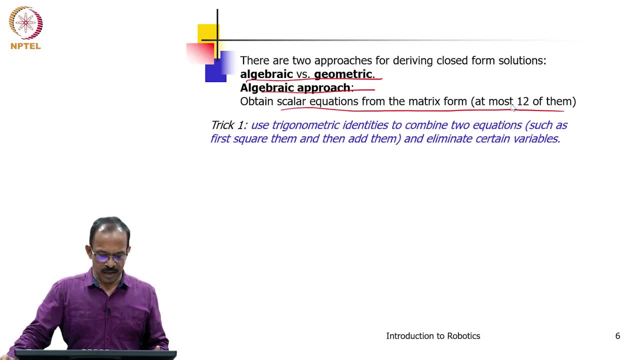 solve them. That is the algebraic approach And in this, so this geometric approach we will not be discussing, because geometric approach normally more of a graphical approach. So you know the position and orientation to be reached and you know the link, length and other orientation, other parameters. 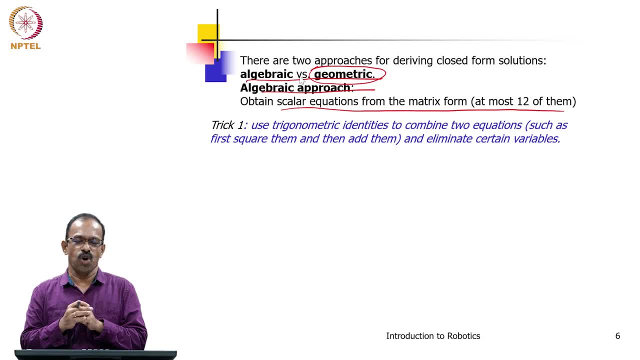 That is the algebraic approach. Okay, So you try to geometrically construct the manipulator position and orientation to see what position or in position of these joints will actually reach the required position, and then find out the joint angles corresponding to that. So we will not be going to that part. we will be looking only at the algebraic approach. 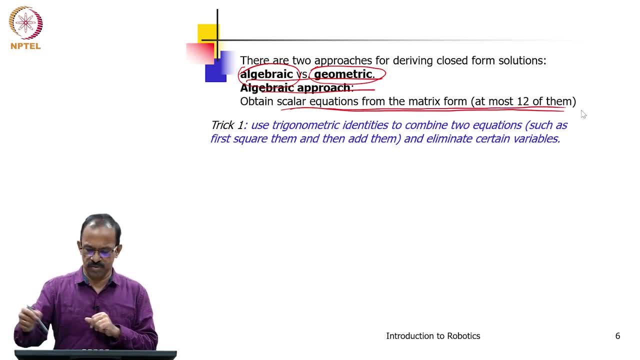 So here we do this by getting the scalar equations from the matrix form. So, as I mentioned, There will be 12 equations, So we can actually write down 12 equations using the matrix, that is, the arm matrix. Now, these 2, 12 equations, always in the- I mean they are all non-linear equations and 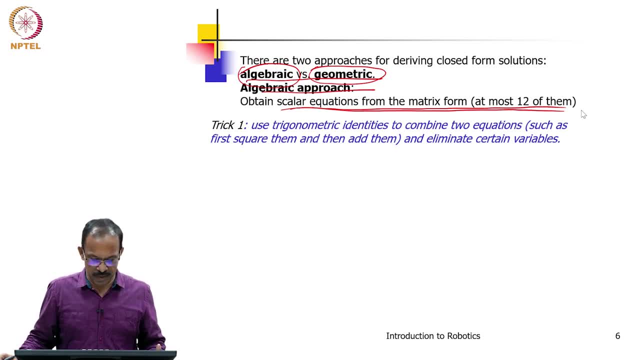 it consists of trigonometric identity parameters and therefore we need to use some tricks to solve them, So they cannot be solved very easily. There are a lot of difficulties in solving this. Okay, There are a lot of difficulties in solving these 12 equations. 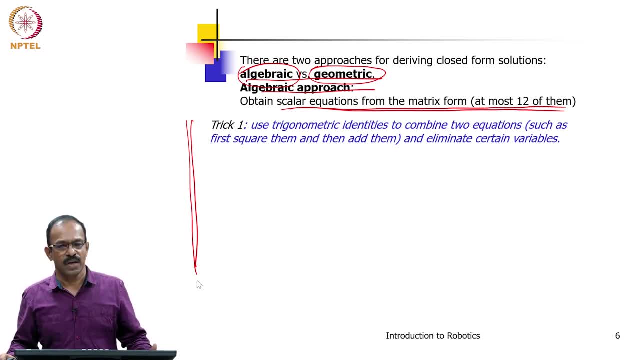 So we use some trigonometric identities to combine 2 equations, first square them and then add them and then eliminate certain variables. So there are different tricks to be used. For example, you have something like a cos theta plus b sin theta, and then so you can. 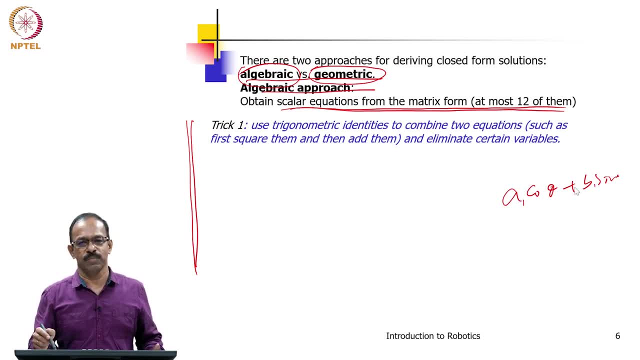 a1, b1, like this, and then probably you can actually, when you add them, cos square theta plus sin square theta will come, and then you will be able to eliminate some of these parameters. There is no problem with that, Okay. Okay, That is what actually says so, such as first square them and add them and eliminate certain. 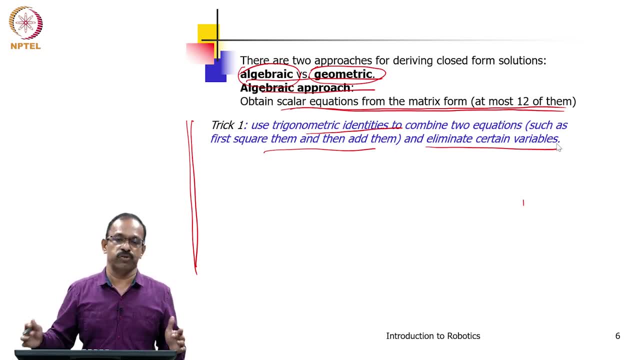 variables. So the trigonometric identities are like sin square theta plus cos square theta is equal to 1.. So such trigonometric identities can be used and we can actually get them by combining equations. So you square them, add and you will get this, and then you can eliminate some of the variables. 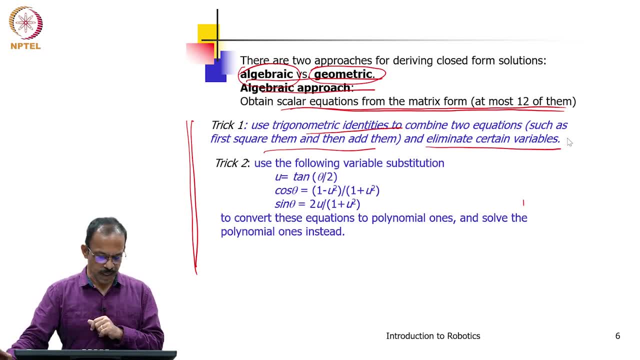 That is the trick 1 we can use, And then the trick to be used is that you use the substitution. Okay, Okay, Okay, So you can substitute for these trigonometric variables with some other and then convert them into polynomials. 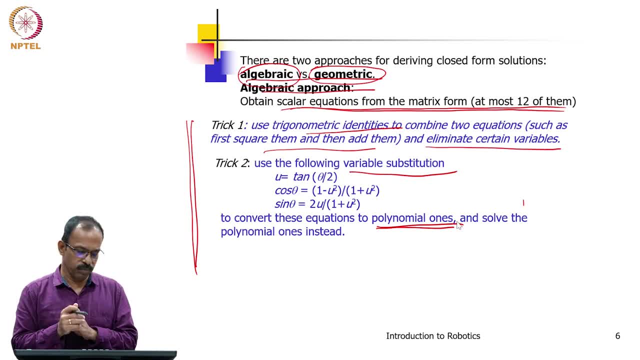 So the trigonometric equations can be converted to a polynomial and then solve the polynomial. that is another way to solve it. So for example you substitute u is equal to tan theta by 2, then cos theta can be written as 1 minus u square by 1 plus u square and sin theta can be written as 2u by 1 plus u. 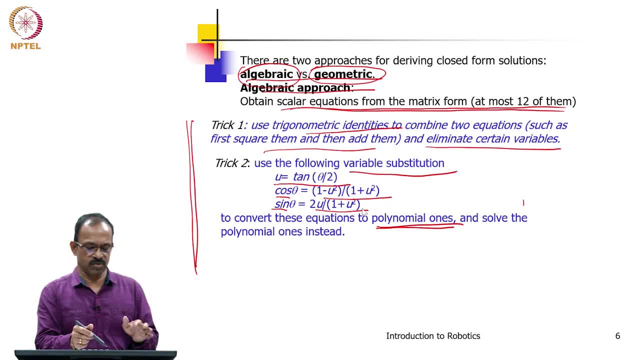 square. Okay, So here the cos, theta, sin theta is coming. you substitute these parameters, these values, and then convert that into a polynomial equation and then solve the polynomial and then get the theta. So finally, we need to get the theta. 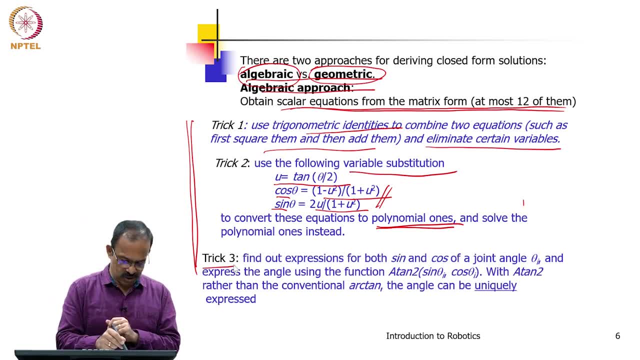 That is the trick 2.. And then another trick to be used is that find out the expression for both sin and cos of a joint angle, theta. So you write sin theta. you find out what is sin theta. Suppose you want to sin theta. 1 is equal to k. 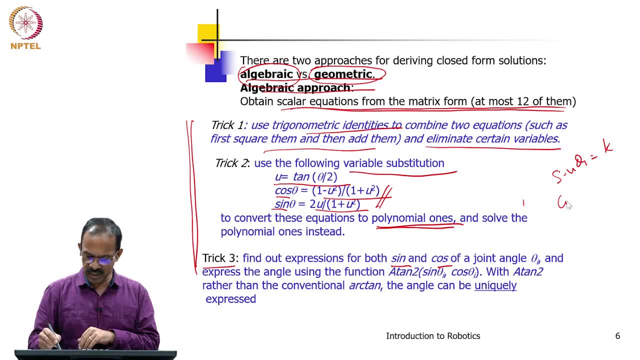 Okay, So sin theta 1 is equal to k, and then you find out cos theta 1.. So cos theta 1, you try to write it as square root of 1 minus k square, so that will be cos theta 1.. 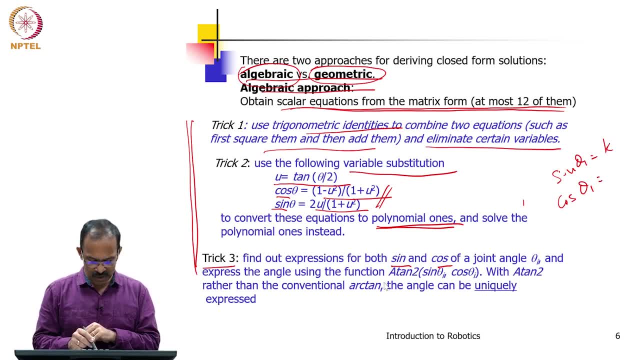 So you have sin theta 1 and cos theta 1 and then use a function called a tan 2 to get the theta value. So a tan 2 cos sin theta, cos theta. So we write it as a function called a tan 2 function. 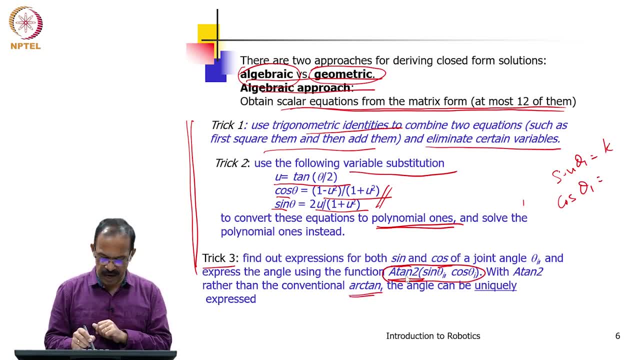 Normal arc tan is not a function. Okay, So normal arc tan is not used, but instead you use a tan 2 function And that can actually give you a unique expression for theta. So when you use the normal arc tan, so theta can actually be anywhere here. 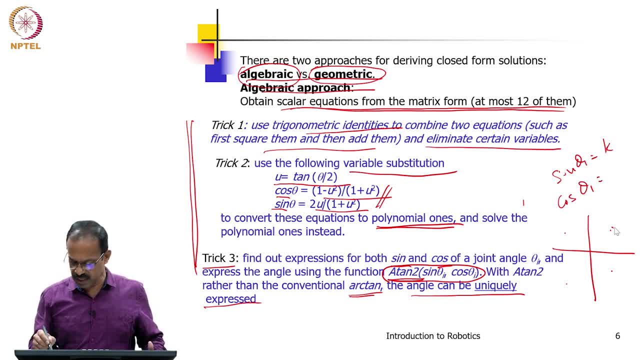 But then when you use an arc tan, it will not clearly tell in which quadrant it lies, because arc tan value will be the same but the quadrant will not be specified. But if you use an arc tan 2 function, a tan 2 function, you will be able to clearly tell. 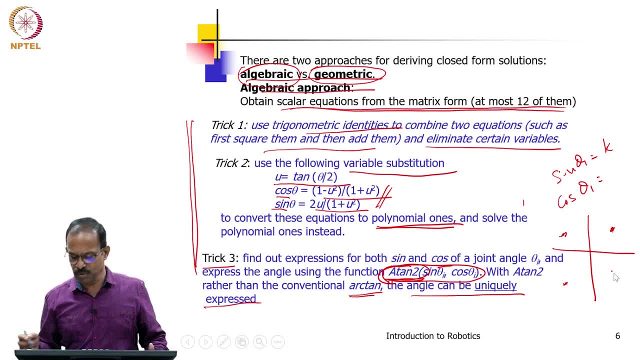 which quadrant it lies, So you will be able to get the theta value uniquely. Okay, Thank you. So this is how we define using arc tan 2 function. I will explain this when we consider the examples of how to use the arc tan 2 function. what? 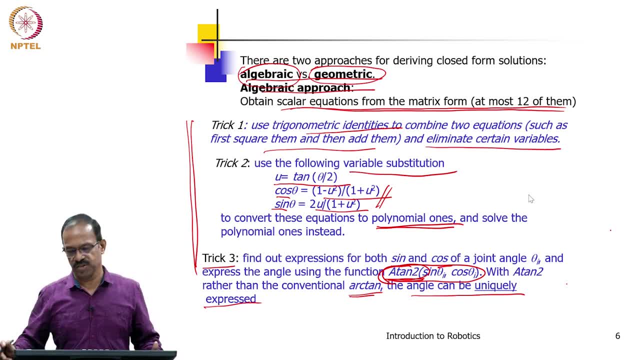 is the importance of arc tan 2 function in solving these equations. So to solve this equation, we need to use some of these trigonometric identities or trigonometric tricks, which actually helps us to simplify the equations and then solve them without much of difficulty. 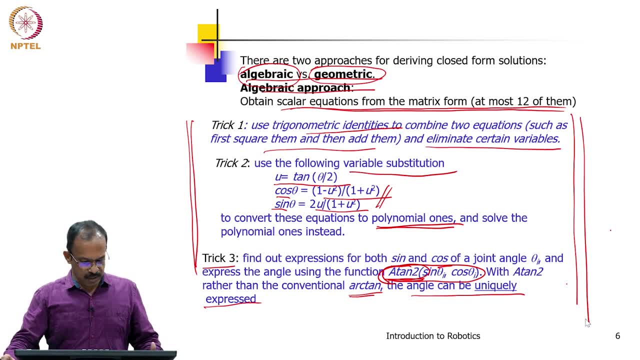 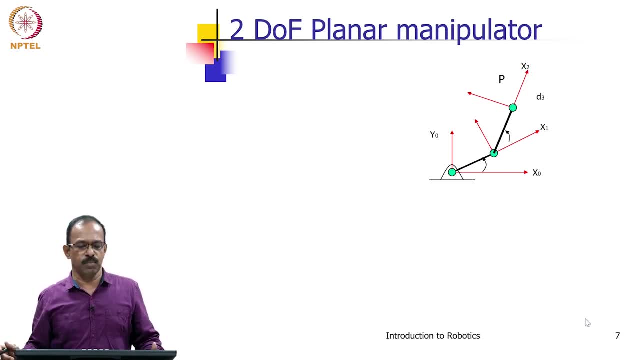 So that is about the method or the way to solve the thing, the inverse problem. So let us take a very simple example of a 2 degree of freedom planar manipulator. So this planar manipulator is given with a link length L1 and a link length L2. we will 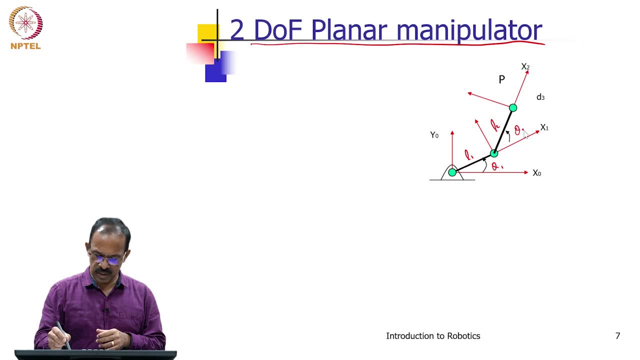 say: And this one is assumed that this one is theta 1 and this one is theta 2.. And this one is theta 2.. And this one is theta 1. And this one is theta 2.. So, as I mentioned the first thing to, in order to solve there for the inverse kinematics, 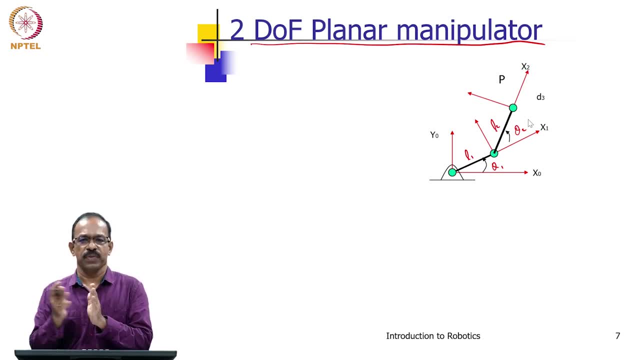 we need to have the forward kinematics relationship and that will give you the a matrix. So we will do the same process: we assign the coordinates around x 0, y 0, x, 1, y1, x, 2, y to x, etc, And then see how to get the forward kinematics. 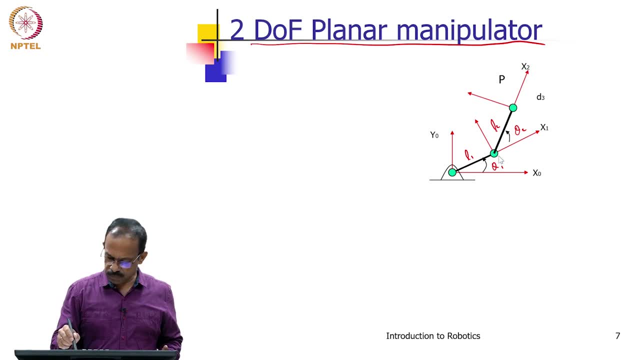 So okay. so now we need to get this forward relationship. So let us write this here. Okay, take this as a Px, Px1 and this is for. so the Px is actually this one. So this is the Px and then this is the Py. So this being a simple two degree of freedom, planar manipulator. 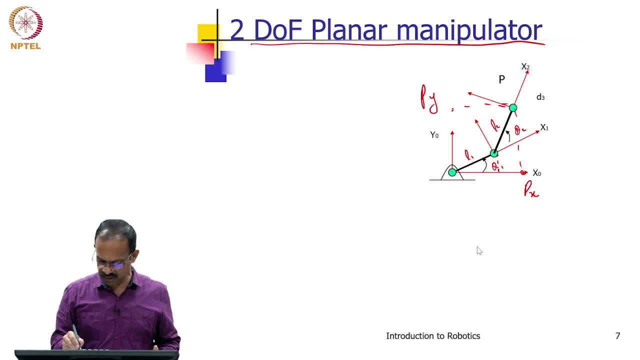 will be able to write this Px and Py very easily. So Px can be written as l1 cos theta 1 plus l2 cos theta 1- 2.. Similarly, Py can be written as l1 s1 plus l2 s1- 2.. 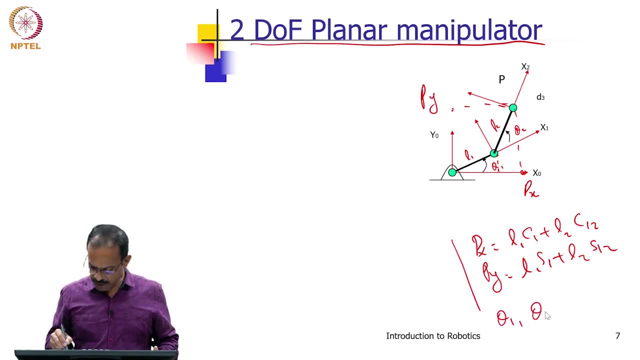 Now we need to solve for theta 1 and theta 2.. So we need to find out for any value of Px and Py. how can you get theta 1 and theta 2.. So that is the position part We are looking. 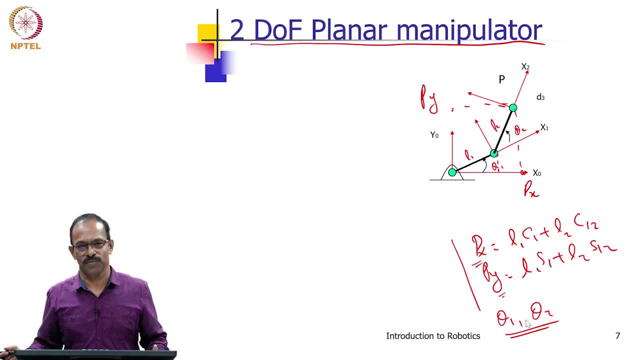 only the positioning part here, just to give the feel of how do we solve it. So theta 1 and theta 2 is to be solved. So here is equation 1 and this is equation 2.. Now how do we solve for theta 1 and theta 2, because we have only these two equation. 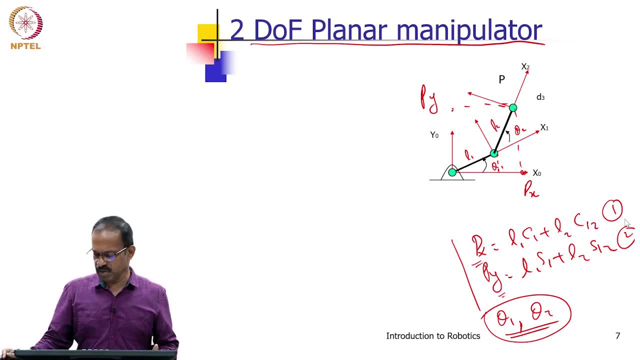 l1 c1 and l1, l2 c1, 2, l1 s1 plus l2 s1, 2.. So what we do, we will try to see some of the. we will try to use some of the tricks to solve this. So one of the tricks is basically: 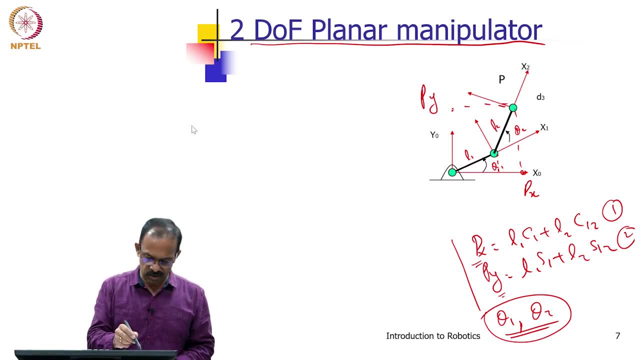 to square and add these two equations. So if I write down as Px square plus Px square plus Py square, So if I square and add them, then I will be able to write this as, like this: Px square plus Py square is equal to l1 square plus l2 square plus 2, l1, l2, c2,. 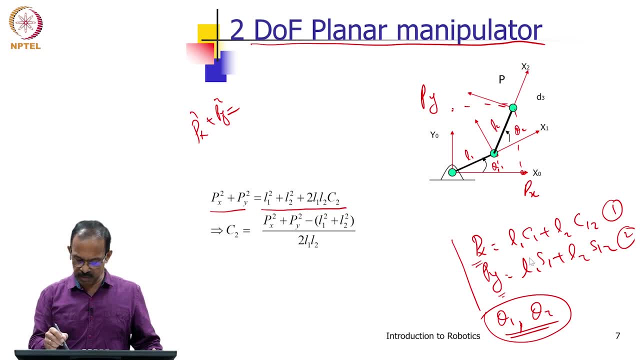 because l1 c1 square and l2 c1, l1, l1 s1 square will actually become l1 square and similarly get l2 square plus 2 l1- l2- c2.. And we can get c2 as Px square plus Py square minus l1. 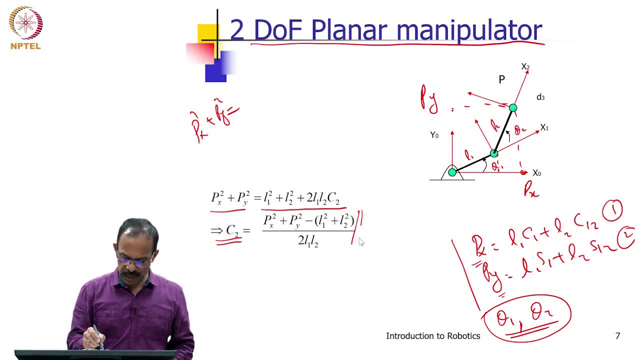 square by l1 square. So that is how we solve this. So we are going to solve this. So L2 square to L1 L2.. So we have solved for C2.. So once we have C2, we can find out theta. 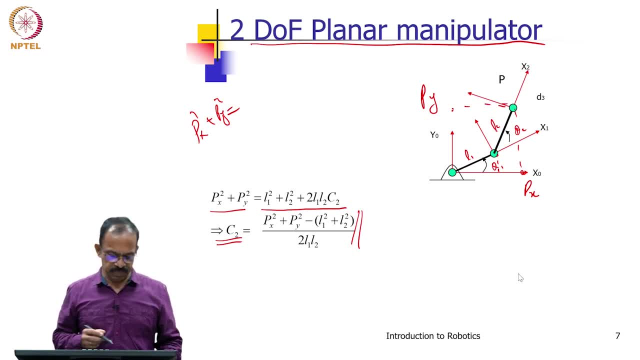 2, we need to find theta 2.. So instead of using directly cos inverse, we do not use a cos inverse to get theta 2, because that will not tell you in which quadrant the theta lies, because at the four quadrants we want to clearly get which quadrant theta is lying. 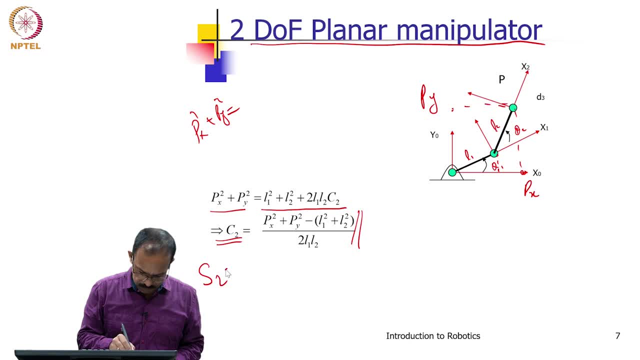 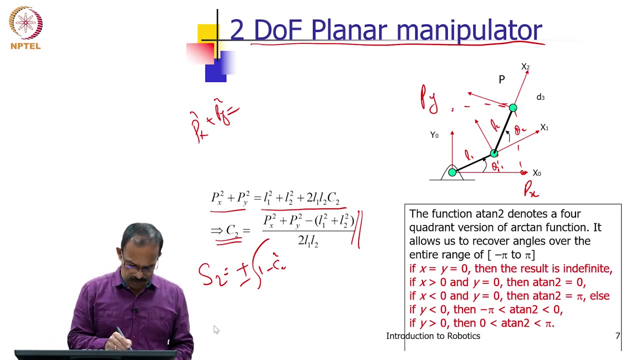 And therefore what we do. we will try to find out S2 from here. So S2 can be obtained as square plus or minus square root of 1 minus C2 square. That is the way how you can get the S2.. And once we have S2 and C2, then we get theta. 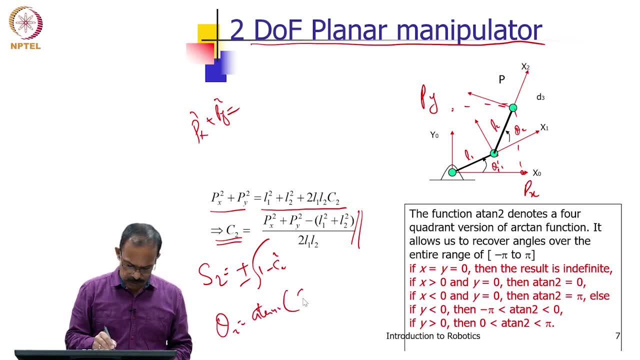 2 as eta n2, S2, theta n2.. So this is the way how we can get theta 2.. And why we are doing this? because, as I mentioned, the function eta n2, eta n2 denotes a four quadrant version of arc tan function. It allows: 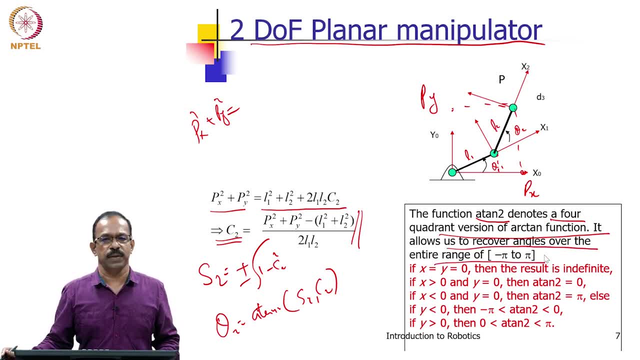 us to recover angles over the entire range of minus pi to pi. So it will clearly tell between pi and minus pi what is the value And how is it doing this eta n2 function? So if suppose it, eta n2, x, y, 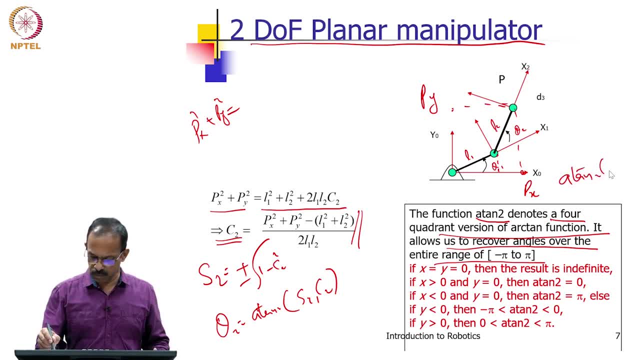 So if you take eta n2, x, y, So it will look at the values of x and y and then decide which quadrant it lies. So if x and y are 0, then it is indefinite. x is greater than. 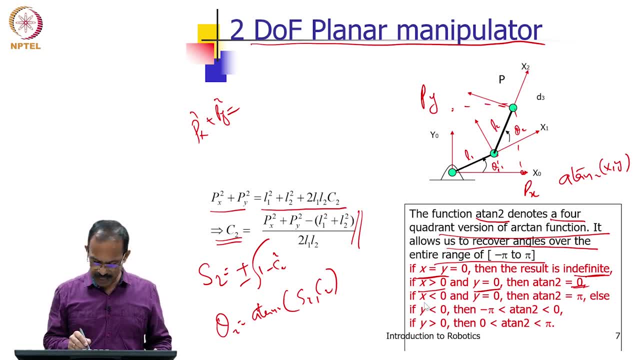 0, y is equal to 0, then eta n2 is 0.. Then x greater than less than 0,- sorry, yeah, less than 0- and y is 0, then eta n2 is pi, And if y is less than 0, then minus pi. So it: 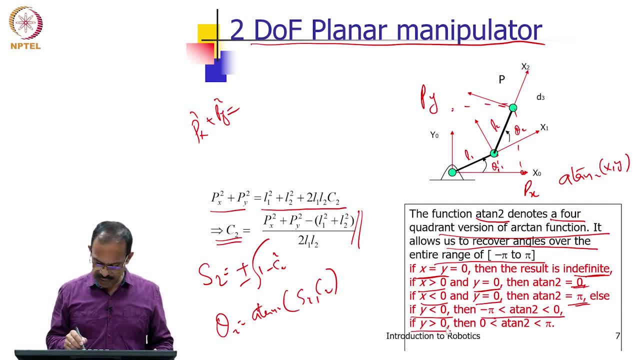 eta n2- 0, it lies between 0 and minus pi. if y greater than 0, then it is between pi, n, 0 and pi. So this way it clearly tells you which quadrant it lies between: 0 and minus pi or minus pi, 0 and pi, or 0 and minus pi. So this way you will be able to get the theta. 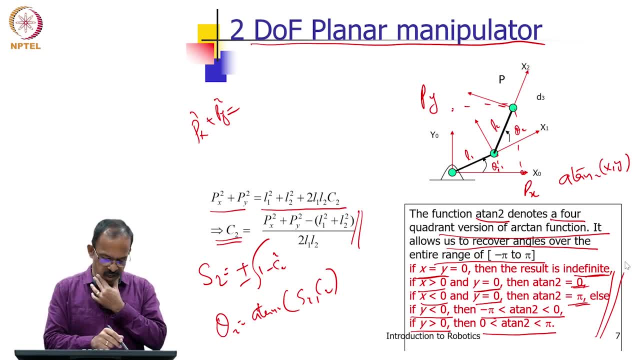 clearly defined within this 4 quadrants. So that is why we go for eta n2 function instead of going for a cos inverse or sin inverse or simple eta n function. So this is the way how we need to get theta 2.. So we will get theta 2 using the eta n2. 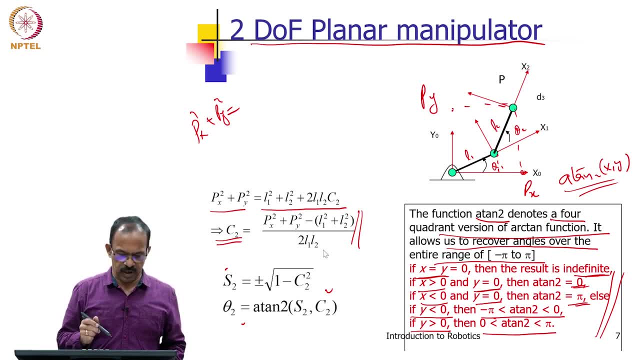 function. So S2 is plus or minus square root of 1 minus c2 square and theta 2 is eta n2, S2, c2.. And now we can see, because there will be two values for S2, you can get two values. 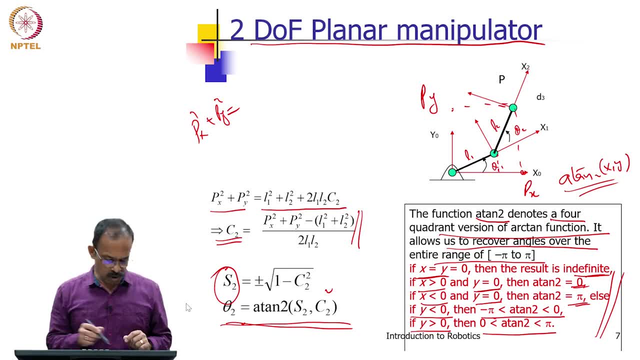 for S2.. So one is for plus and one is minus. Now you will be getting theta n2.. Two values for theta 2 also. you will get theta 2 for one value of S2 and theta 2 for another value of S2.. Now, if both the values are actually lying within the join limits, 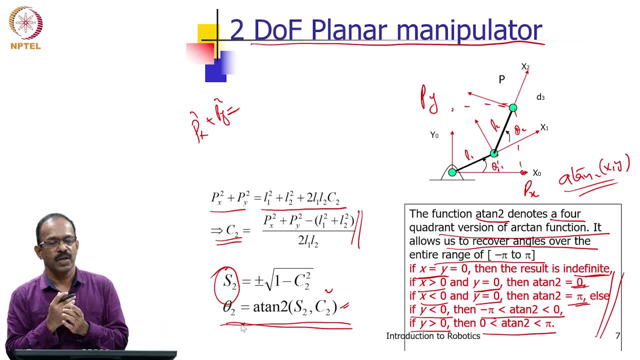 of the manipulator, then you have to take both the values as a solution, And if one is outside the join limit then you can eliminate and then proceed to select the find the next join angle. But if both are in the join limits, somehow both happens to be in the join limit. 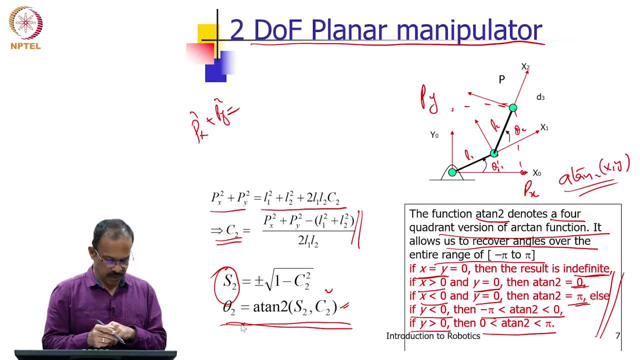 that shows that there can be two ways- theta 1 value and theta 2 in this case, And you have to use both the values for solving the next join angle. So you will be getting multiple solution that way. So that is, how do you get who? you get the theta 2.. 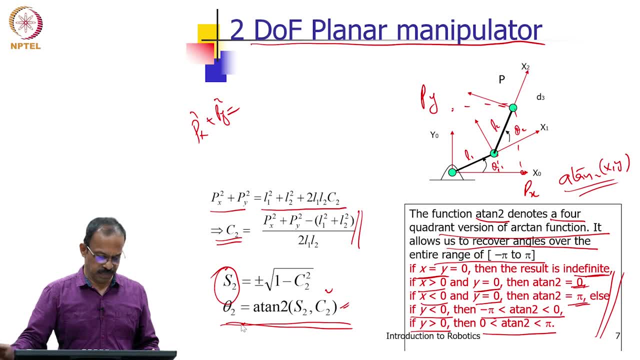 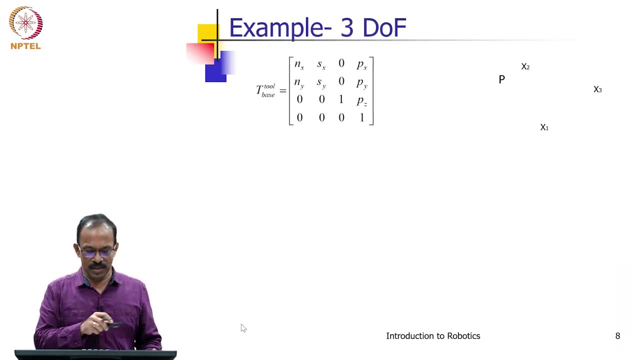 Now you need to solve for theta 1.. So you have to substitute for this px value px L1, c1 plus L2 c1 to that relationship and then solve it for the join angle next join angle. So we will take a more complex one and then go to the solution. This one I just want to. 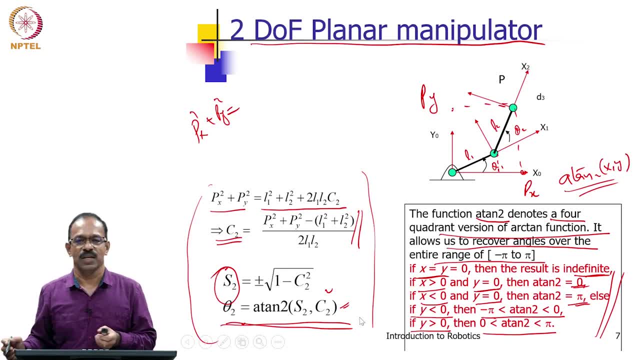 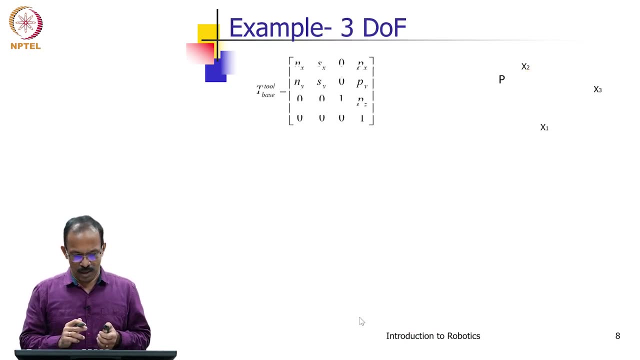 tell you how do you use the tricks to solve for the joint angles. So we will see look at the solving for theta 1 and other join. if you have more joined angles, how do you solve? So we will take more complex problems and then try to solve it. So this is the 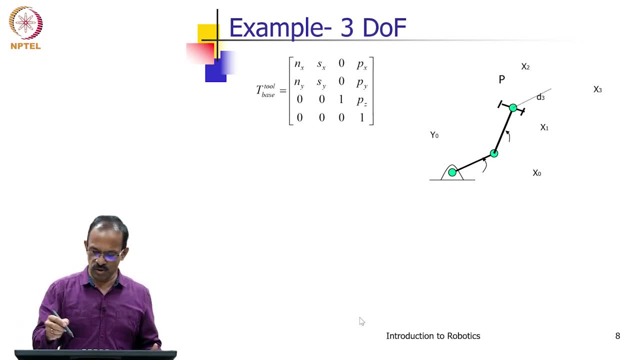 three random case. so we assume that there is another joint here. it is actually projecting out in, this manipulator is projecting out from the plane and with the distance d3. and then you have this other joints 1, 2 here, joint 1, joint 2 and you have another joint 3.. 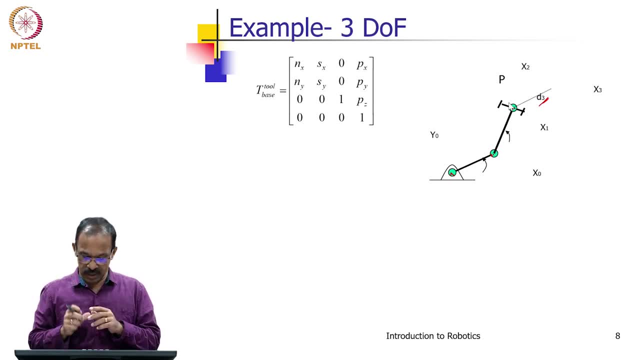 So here, since it is projecting out and there is no other thing, so the orientation will be given by this. so always, the axis is always vertical. So you will be having Nx, Sx, Ny, Sy and 001, 001 as the orientation matrix, the orientation. 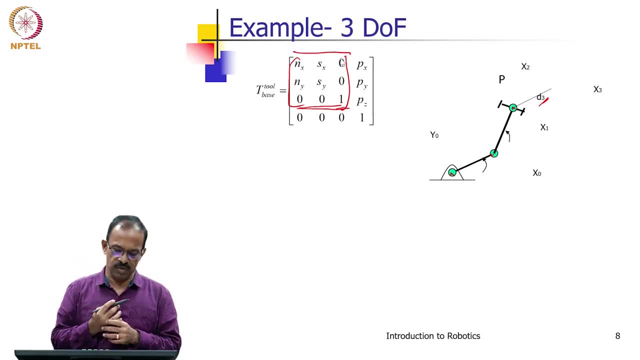 of the tool will be always in this format: Nx, Ny, Sx, Sy, and the position will be Px, Py, Pz. So Px Py is the position. this Pz is because of the d3 which is projecting up. 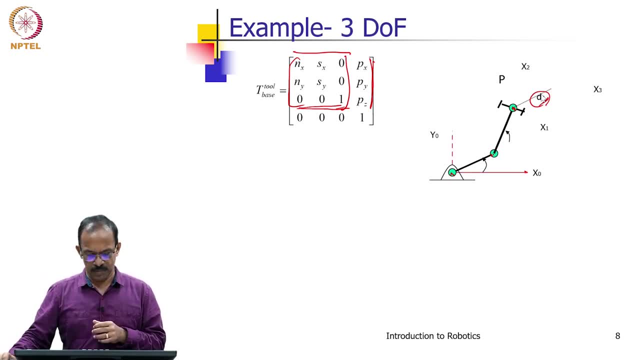 Now, if you have to solve this problem, We will see so. first we will assign the coordinate frame x0, y0, x1, y1 and x2, y2, and then tool tip will be having the final coordinate position, x3, which is actually projecting out. 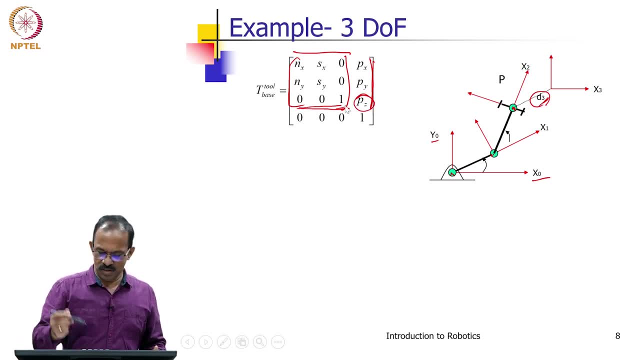 So you can see Pz will be always d3 because it is projecting out and then it is actually rotating, so it will be d3, distance Pz. So you can actually find out the parameters here, The dh parameters. so first we need to solve the forward kinematics. 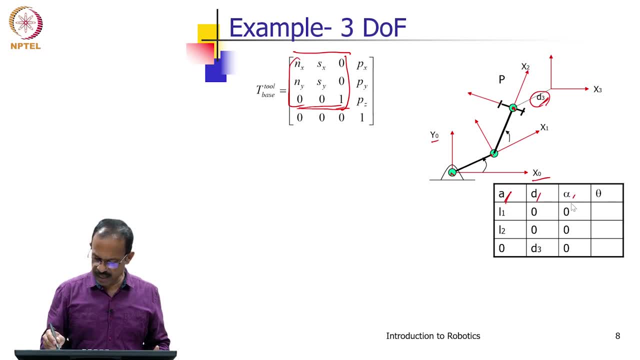 So to solve the forward kinematics, we will find out the parameters a, d, alpha and theta. So here this: l1, l2 is a and d3 is. this is 3 and then alpha is 0, because all the joints are axis, are parallel and theta is a variable. so theta1, theta2, they are variables. 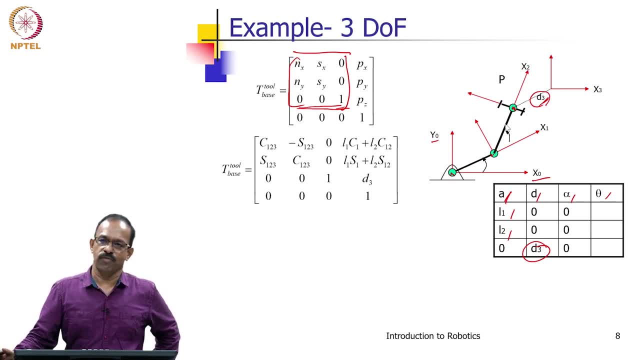 Okay, Now if you write this forward relationship using the transformation matrix, you will be able to find out the forward relationship or the arm matrix. it will be like this: So your Px will be l1, c1 plus l2, c12, as we saw in the previous case. also, Py will. 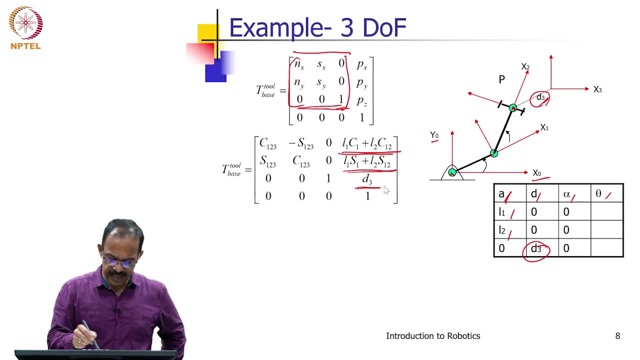 be l1, s1 plus l2, s12 and Pz will be d3. So this will be the position vector for the tool or this coordinate frame. position will be given by this relationship: l1, c1, l2, s2, l1, s1 plus l2, s12 and d3. 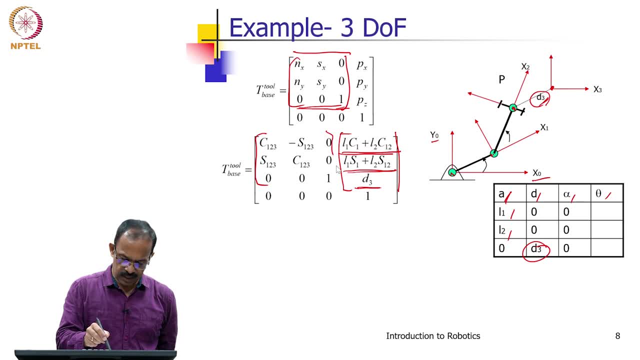 Now the orientation will be given by this 3, the matrix c123 minus s123, s123, c123, 001.. Okay, And you have this. 3 equation: Px, Py, Pz and Nx, Ny, Sx, Sy. 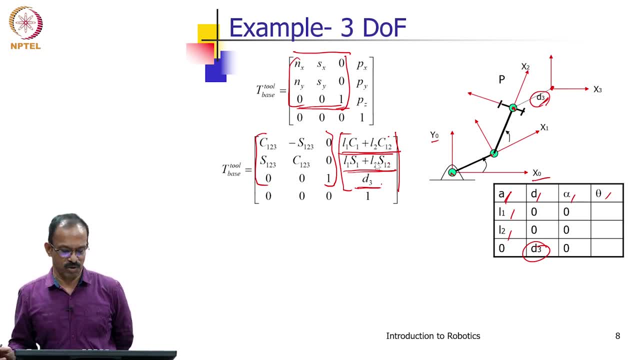 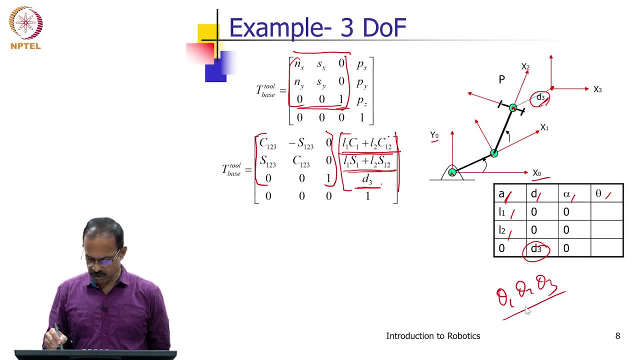 Okay, Okay, Okay. So this is theta 1, theta 2 and theta 3.. You need to solve for theta 1, theta 2, theta 3.. So you have this 3 equation plus 2 equations here. 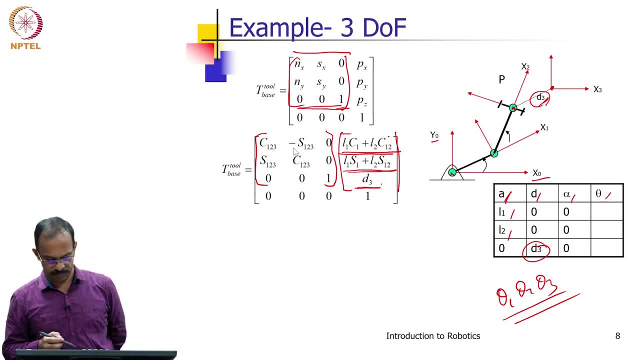 So 5 equations are there, So we can actually solve it easily. And we will write this one relationship now, So Px. we will write: Px is equal to this, Py is equal to this, Pz is equal to this. And then we will write: Nx is equal to C123. 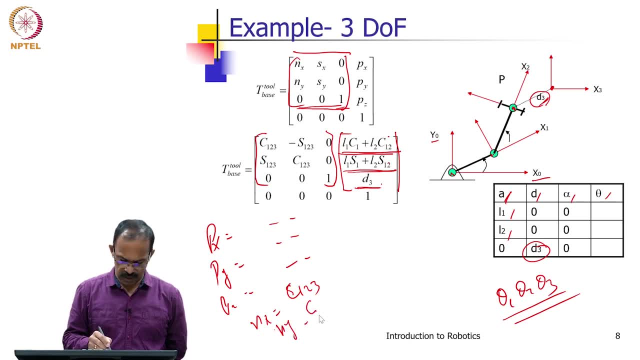 3, n. y is equal to s 1,, 2,, 3, etc. And similarly s x is equal to minus s 1,, 2, 3,. s y is equal to c 1,, 2, 3.. So this way we will write this relationship and then we will try to solve. 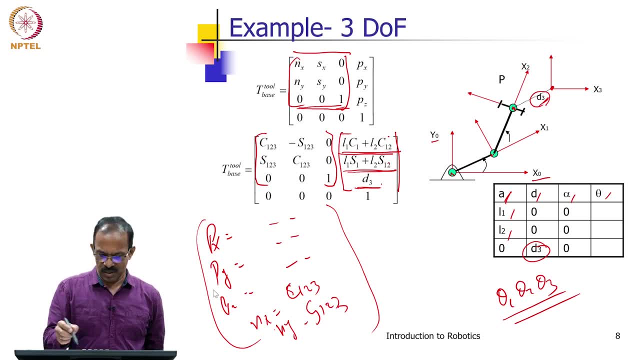 it. So, as we saw in the previous case also, so p x will be getting l 1, c 1 plus l 2, c 1, 2, p y is l 1, s 1 plus l 2, s 1, 2.. So if you square and add them, you will be able. 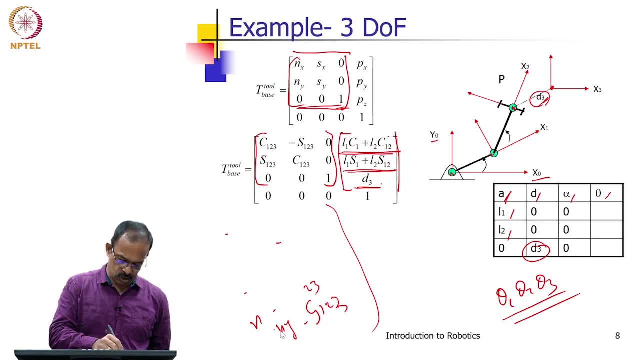 to get theta 2.. So theta 2 can be solved, And so theta 2 can be solved using this method, and then theta 1,, 2,, 3 can be solved using this relationship, because you have c, 1,, 2,. 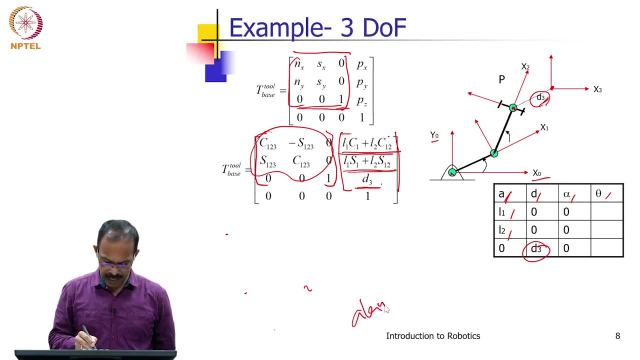 3 and s 1, 2, 3.. So you can actually use that to find out a tan 2, c 1, 2, 3 and s 1, 2, 3, you will be getting theta 1, 2, 3.. So theta 1, 2, 3 can be solved and theta 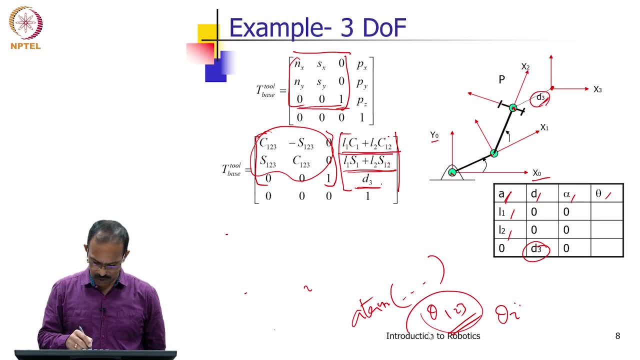 2 can be solved, c 1,, 2, 3.. So theta 2 can be solved directly from here and theta 1,, 2, 3 can be solved from here. That we saw how to get theta 2 in the previous case and theta 1,, 2, 3 can be easily solved. 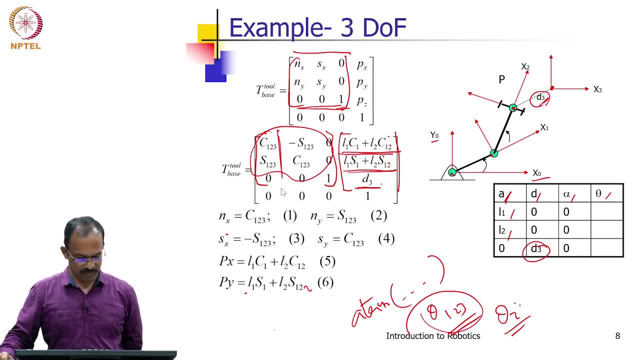 from here. Now the question is: how do you get 1 and 3?? So these are the relationship you have: n x s x, n y s y and p x p y. So we have these 6 equations written here Since. 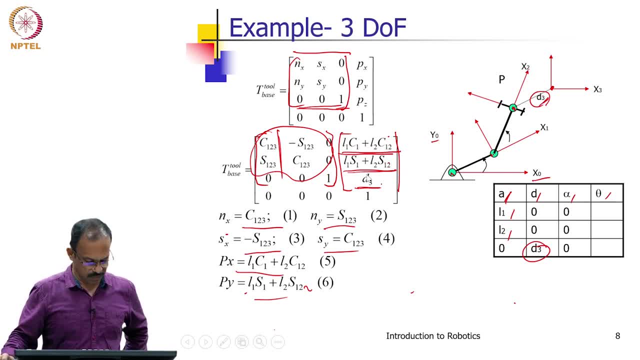 p, z is equal to constant. we did not write that as a separate equation. Now, squaring and adding 5 and 6, we get theta 2.. So we know c 2 can be obtained and by using the same method that we discussed in the previous example, we can get theta 2 as: 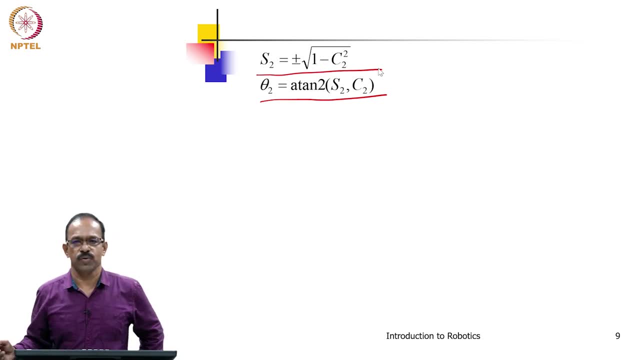 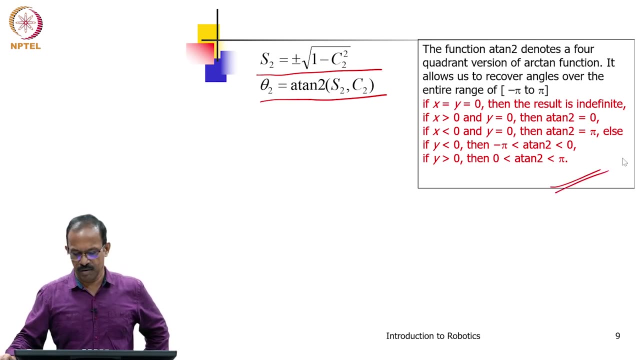 a tan 2, s 2, c, 2.. So theta 2 can be obtained. Now using the other equation we will be able to so this one I already explained. how do we get, how do we use a tan 2, get the theta. 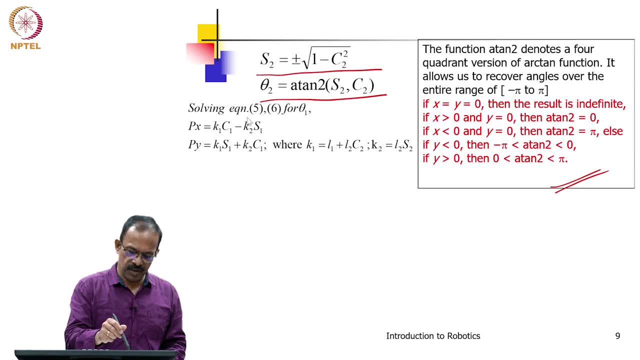 2., 3., 4.. So this is 5 and 6 for theta 1.. So now theta 1 is to be solved, So theta 1 cannot be directly solved, So we need to have a substitution here. So what we do, We do a. 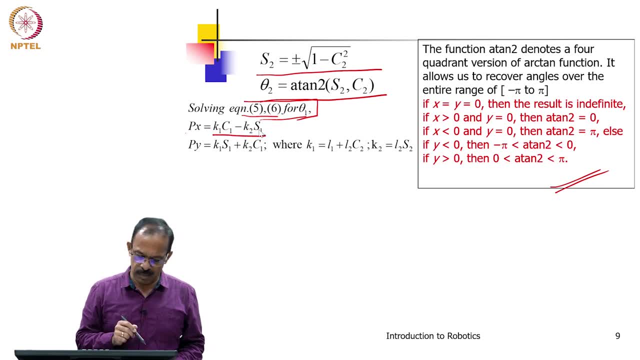 substitution here, saying that p x is equal to k 1 c 1 minus k 2 s 1, and p y is equal to k 1 s 1 plus k 2 c 1, where k 1 is equal to l 1 plus l 2 c 2 and k 2 is equal to l. 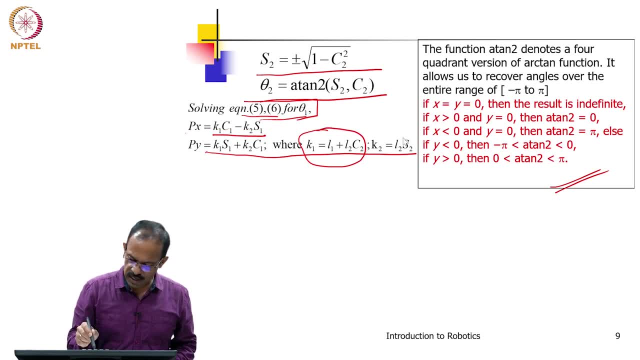 2 c 2.. So if we make a substitution like this: k 1 is equal to l 1 plus l 2 c 2 and k 2 is equal to l 2 s 2.. And when you do this substitution, then we can write: p x is equal to k 1 c 1. 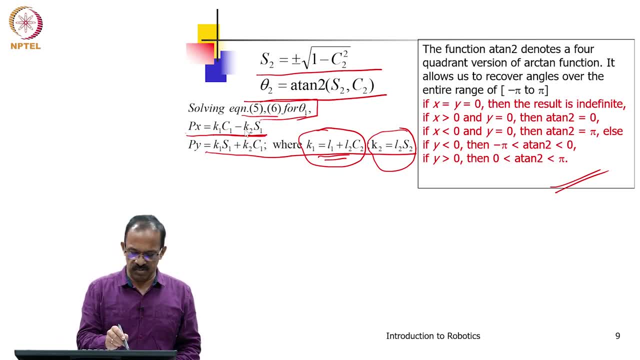 minus k 2 s 1.. So the previous p- x equation can be expressed like this: because of this substitution, And then we write down, we again substitute: k 1 is equal to r cos gamma. k 2 is equal to r sin gamma. 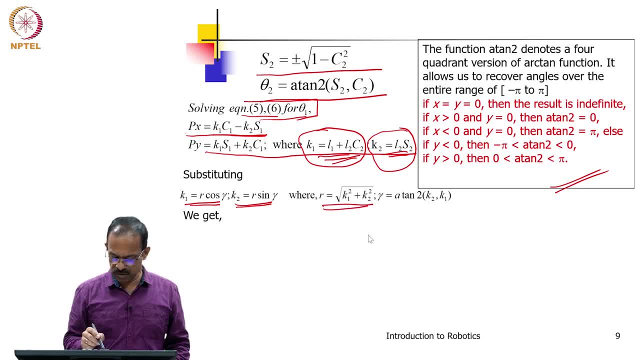 r sin, gamma, where r is equal to k1 square plus k2 square root and gamma is a tan 2, k2- k1.. So this kind of a substitution is needed in order to solve for S1, because we have this, the relationship Px is equal to L1- C1 plus L2, C1- 2, so to solve that one we need. 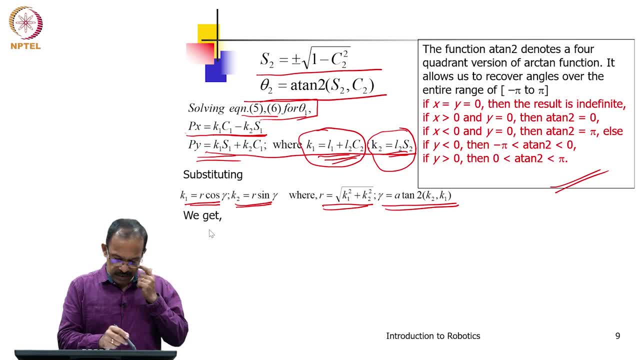 to have a substitution like this, And when you do the substitution we will get it as Px by r is equal to cos gamma cos theta 1 minus sin gamma sin theta 1, and Py by r is equal to cos gamma sin theta 1 plus. 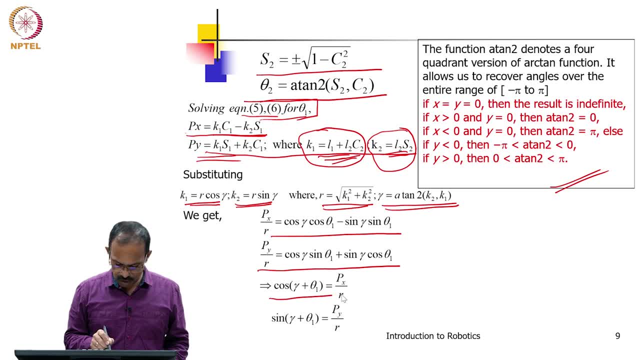 sin gamma, theta 1, and from there we can get cos gamma plus theta 1 as Px by r, sin gamma plus theta 1 as Py by r. And since we know gamma, so gamma is actually given as a tan. 2, k2, k1, and k2 and k1 are known. 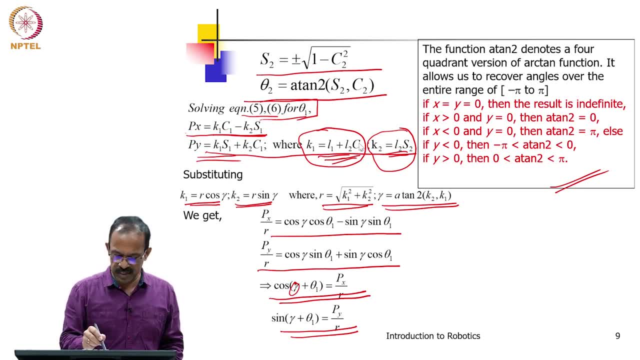 again. So because k2 is known, L2- S2, k1 is L1 plus L2- C2- both are known- we will be able to get gamma, and then we will get cos gamma plus theta 1 as Px by r and then sin gamma plus. 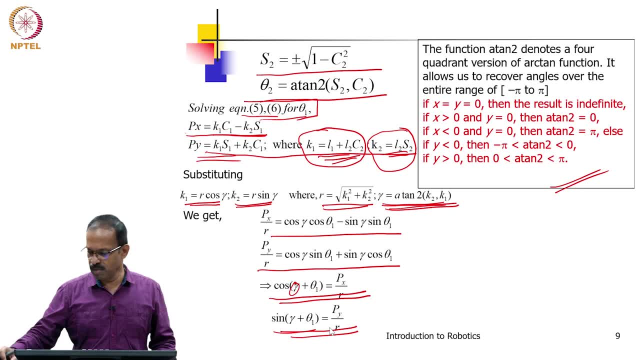 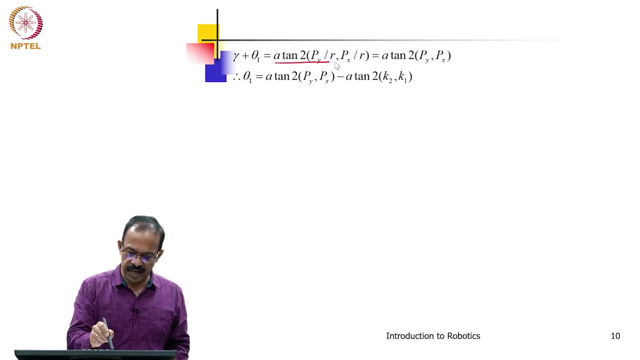 theta 1 as Py by r, And using these two relationship we will be able to get cos this theta 1, as so gamma plus theta 1 can be obtained as a tan 2, Py by r, Px by r, and so a tan 2 is Py by Px, R. 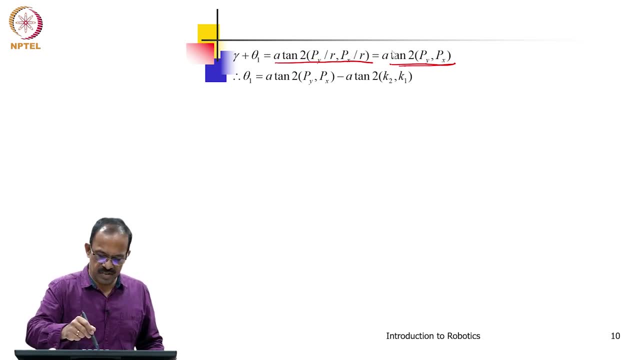 is constant, So you can write. So you can write: gamma plus theta 1 is a tan 2 Py Px and therefore theta 1 is a tan 2 Py Px minus a tan 2 k2, k1, k2 and k1 are known and therefore theta 1 can be solved. 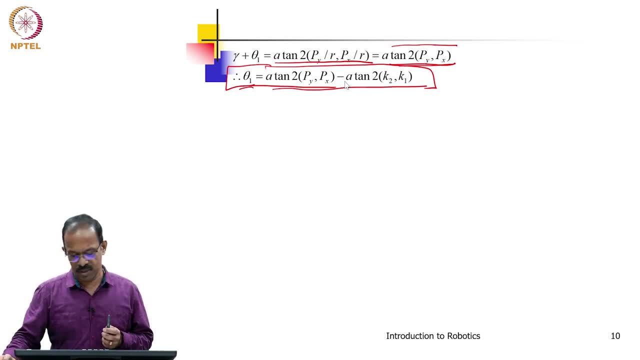 So this is the way how we can get theta 1 solved, And once theta 1 is solved, then theta 2 is already solved and we can get theta 1, 2, 3.. So theta 1, 2, 3 can be obtained as a tan 2 n by nx, as I mentioned, and theta 3 can be obtained.